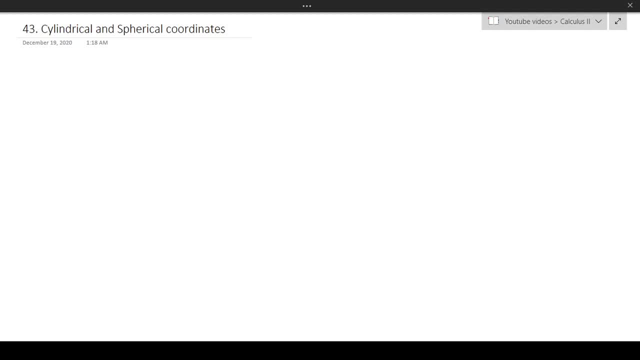 systems in two dimensions. There's many reasons why in 3D surfaces it is necessary to kind of extend our definition of coordinate systems from two dimensions into three dimensions. So, aside from this, we're going to talk about coordinate systems in two dimensions. 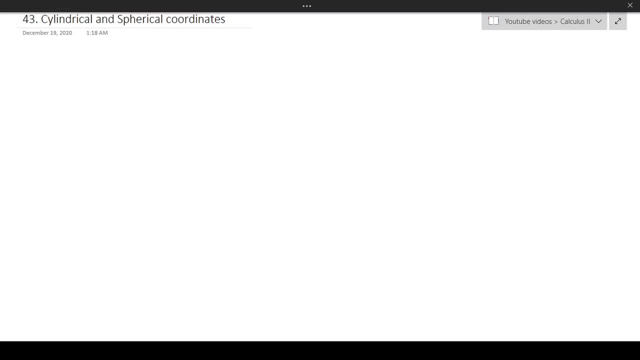 So let's talk about the first one, these kinds of coordinate systems which accounts for the idea that, well, we also have to convert the z-coordinates or the third dimension in some particular way. So how do we do that? So first let's talk about the cylindrical coordinate system. 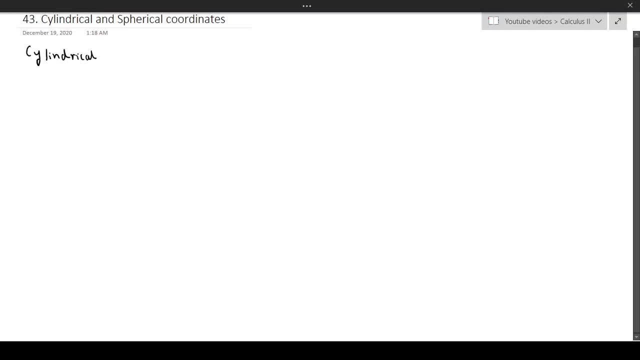 So this is one of the first ways in which we can combine the idea of two polar coordinates and three-dimensional geometrical figures as well. So let's go ahead and do that. So, cylindrical coordinates- Okay. so let's go ahead and underline that. Okay, so let's talk about how to convert. 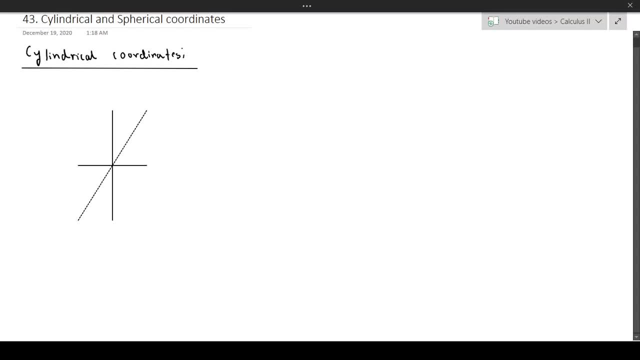 from 2D to 3D. So let's go ahead and underline that. So let's go ahead and underline that. So cylindrical coordinates: Here's a 3D axis of sorts, And then let's go ahead and draw some kind of coordinates. So let's. 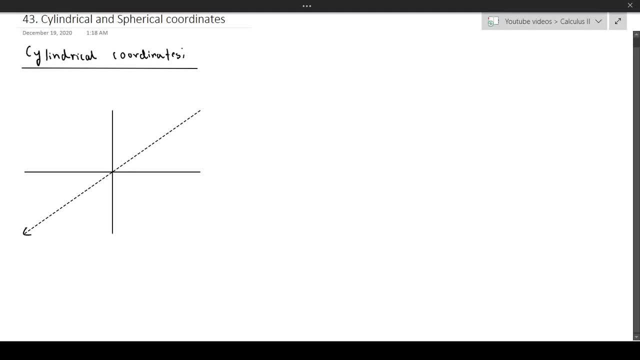 represent this direction as the x-axis. Let's call this the y-axis And let's call this the z-axis, right here. Okay, now let's denote a random kind of point that goes from the origin. So and suppose it goes from the x-axis to the y-axis. So let's call this the y-axis And let's call this the z-axis. 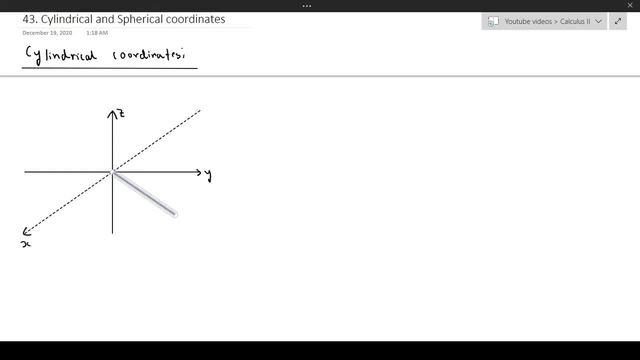 Because it goes this way right there, And let's say we have another point that goes up, So let's say we go up this way. Okay, now let's denote some points. Let's call this O, which will be origin. 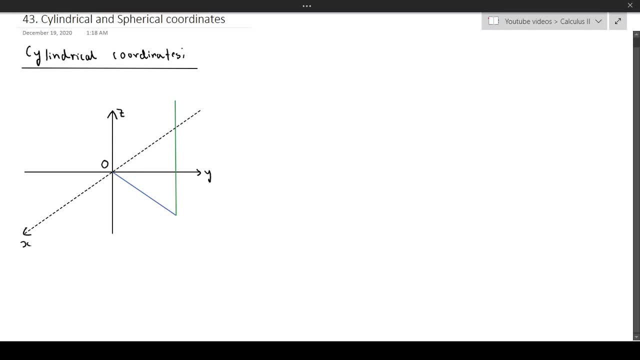 Actually I'm just going to put that here. So that's going to be the origin O, The angle from the x-axis to this blue line. I'm going to call theta, And then let's define this intersection point between the blue and the green points. 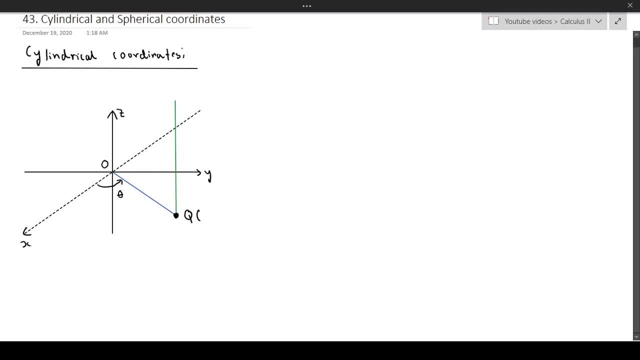 as point Q, which we can denote as R, theta, and 0. and the reason we're saying 0 is because, just to be very clear, that's not the same as this origin. that's wrong. but my point is that this is 0 because the Z coordinate. 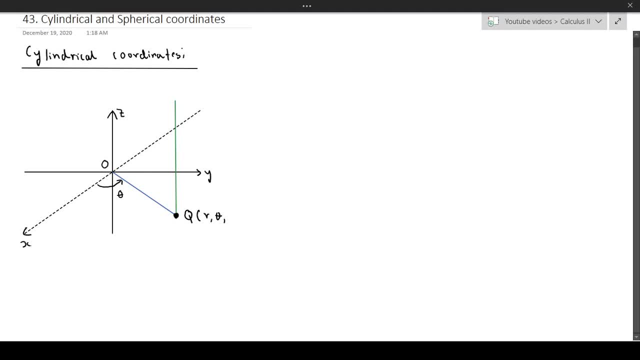 right, there is 0, so don't confuse the two things. in fact, I'm actually going to write 0 and indicate that here I'm saying that Z equals 0, just to be very clear and let's take a look here I'm going to call this point P. 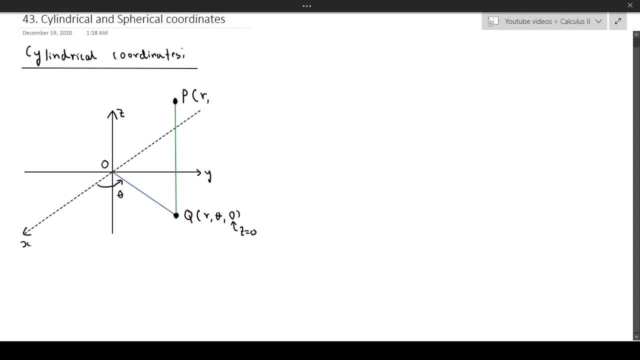 and I'm going to denote these coordinates as R theta, and this time I'm not at Z equals 0 anymore, so I actually have a Z coordinate here. so that's kind of what's going on here. so this is known as the cylindrical coordinate system and it's kind of like the 3D version of polar coordinates. 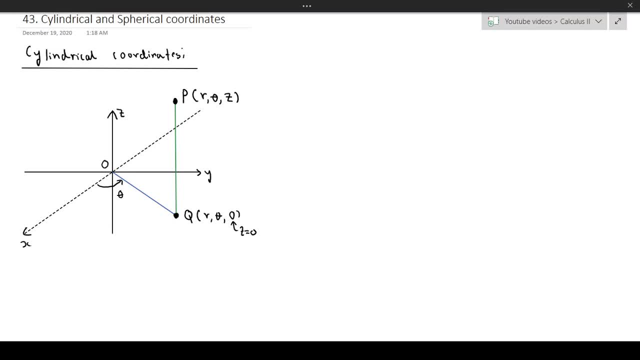 the only difference is that instead of defining X and Y, we also have an extra Z coordinate. so in cylindrical coordinates we have X equals R cos theta, so that's the same as polar coordinates. then we have Y equals R sine theta, that's the Y coordinates. and then we have Z equals. 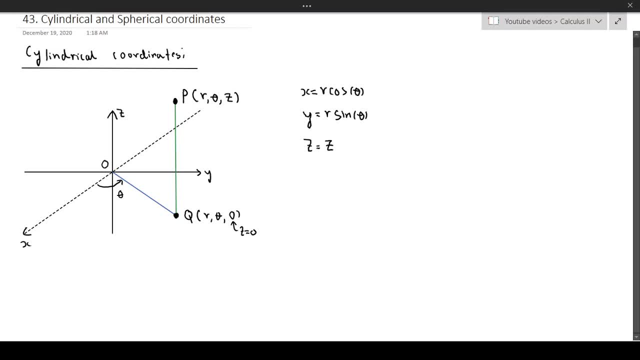 well, just Z. so we haven't really explicitly defined anything per se in terms of change. the only kind of quote-unquote change that we have is that we just define Z as Z, and that's basically the situation. that's going on okay. additionally, we can define a few other coordinates as well. 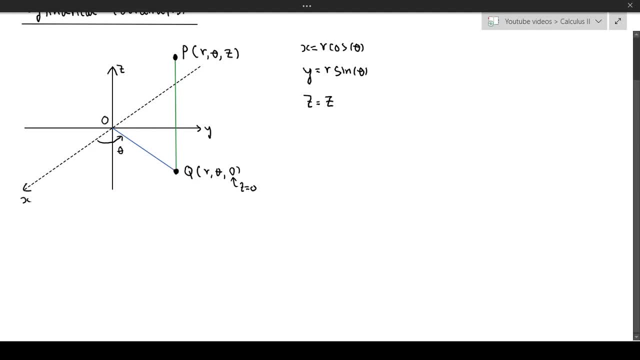 so let's just go ahead and do that. we also know that from polar coordinates, X squared plus Y squared is equal to R squared. and then from trigonometry we know that tan of theta is equal to Y over X, but then this implies that we say that theta 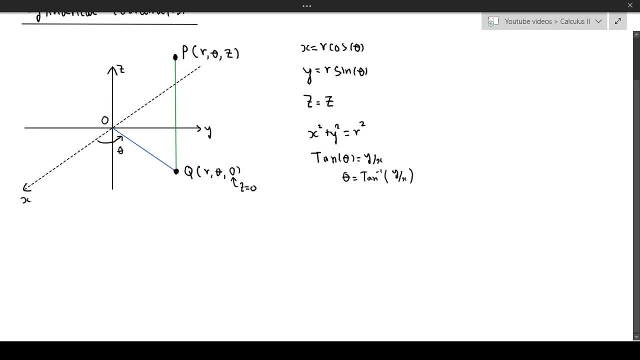 is equal to tan inverse of Y over X, so this way we can get an angle as well. and of course, as you mentioned, z equals z, so there's nothing different about that situation. Okay, now this is good, but this isn't really. 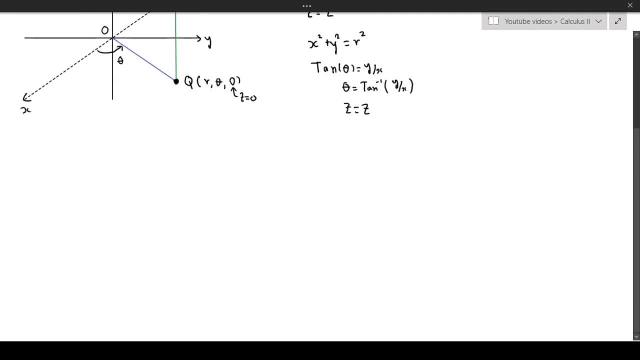 captured the idea of 3D dimensions, and there's a more common kind of system that's used in 3D or vector calculus, and that is the spherical coordinate system. So let's go ahead and denote this coordinate system with this following axis. So I'm going to start with a 3D axis, as normal. 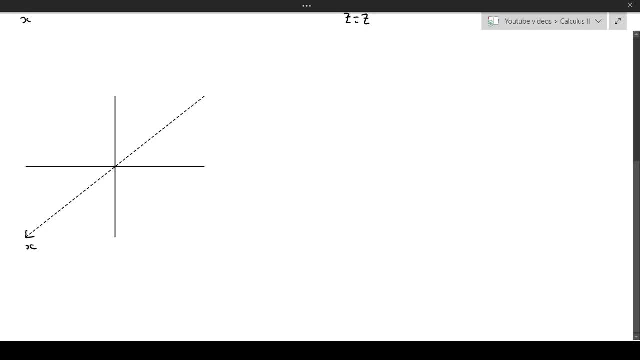 so I'm going to denote this side as the x-axis. I'm going to denote this side as the y-axis, just to be very clear. Yeah, good, And then, as before, I'm going to denote this side as the z-axis. 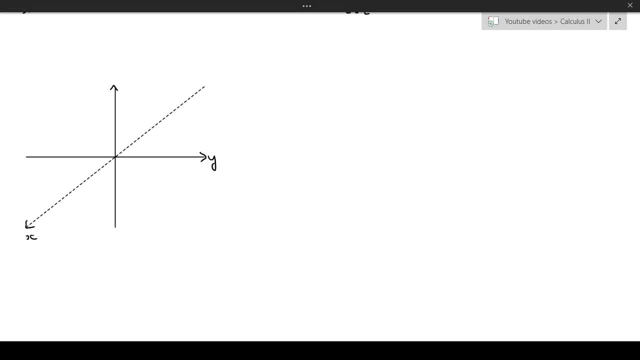 So let me just undo that, Okay, Okay. so it's the same idea This time. I'm going to draw two lines, though One of them is going to be from the origin to some random point in the x-y plane, in the positive x-y plane. 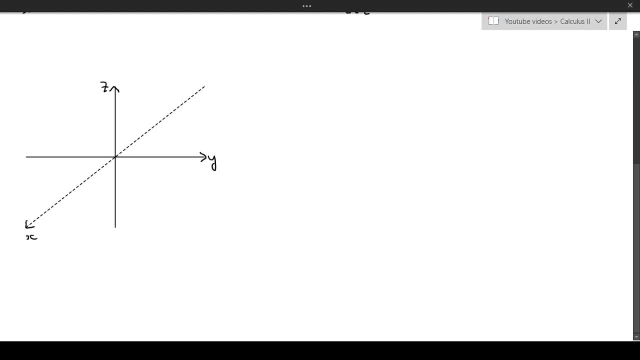 So I'm going to draw that part using a blue line once again. Then, this time, though, I'm going to denote another line going up in the positive z direction, So it's going to look something like this: In fact, I'm actually going to draw that part in green, So let's go ahead and 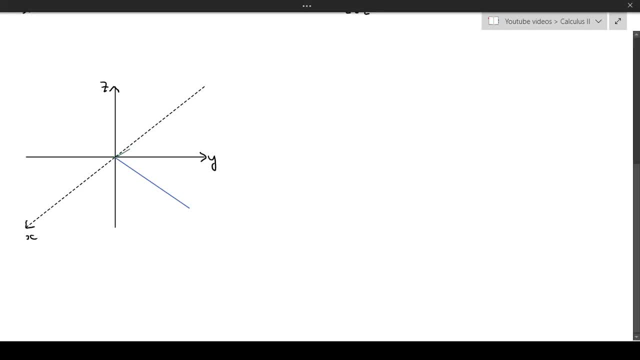 do that, Okay. so here is what kind of what I was interested in, And then I'm going to join these two points using another color, So let's use black again, Okay. so at this point, this is kind of what's been going on. Okay, let's call this point. 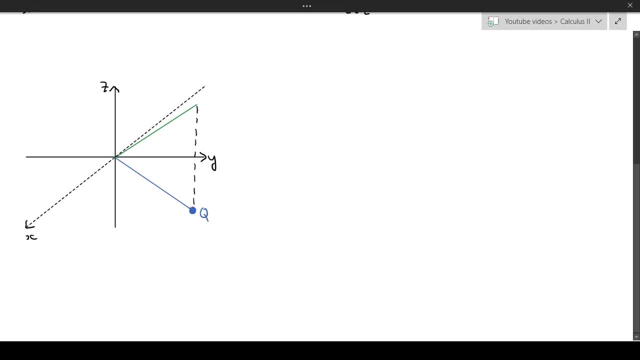 point q, which I'm going to denote, as in fact I'm actually going to write this in black just to kind of emphasize the colors a little bit. So q I'm going to denote this with the following coordinates: this time It's going: 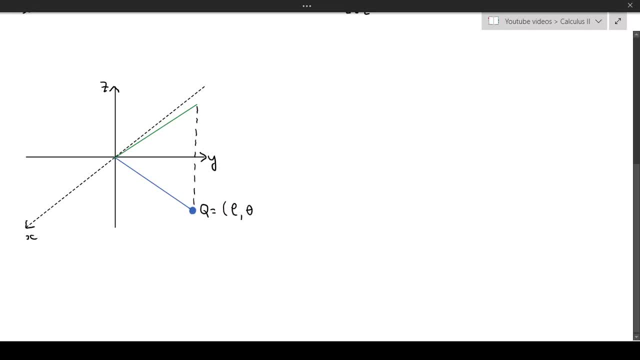 to be rho, the Greek letter rho, theta, and zero once again, because z is zero. So there's nothing special about that, And I'm going to denote this point as p, which is going to be rho theta, and then the angle phi. Sometimes. 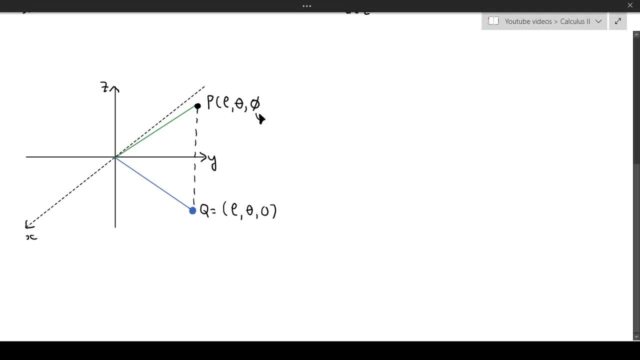 in various textbooks it's written with lowercase phi or uppercase, it doesn't really matter. So another way to write phi is like that, but doesn't really matter. Either one of those are equivalent, Okay, so let's kind of label a few things here, Just like before. this is the angle between the 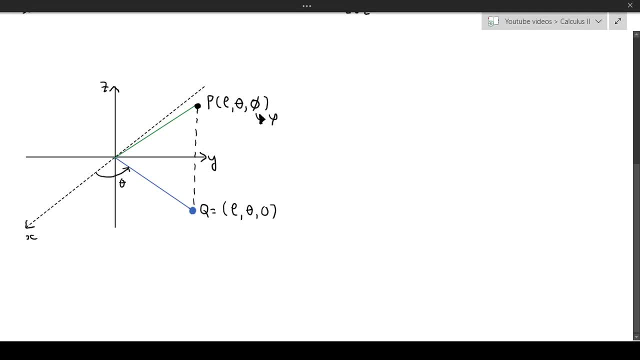 positive x axis and the blue line. that's still going to be angle theta, But this time the group, the length of the green line, is going to be rho, And then the angle from the positive z axis to to the green line. I'm going to call that angle phi. So let's just define a few things, So phi. 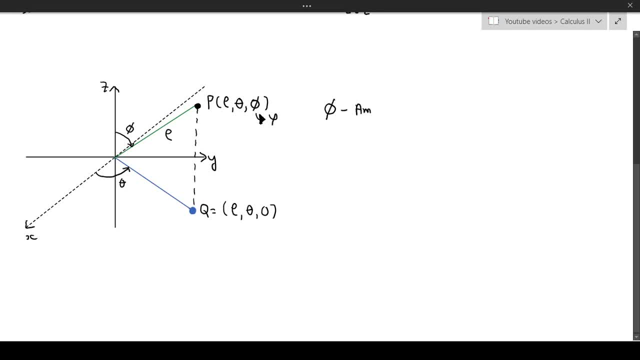 represents the amount of depth, so the angle of the depth. So notice that in terms of depth we only need to go from zero to pi. we don't need to go any deeper than that because that's just physically not possible. If I go over that, we'll actually get less deep. 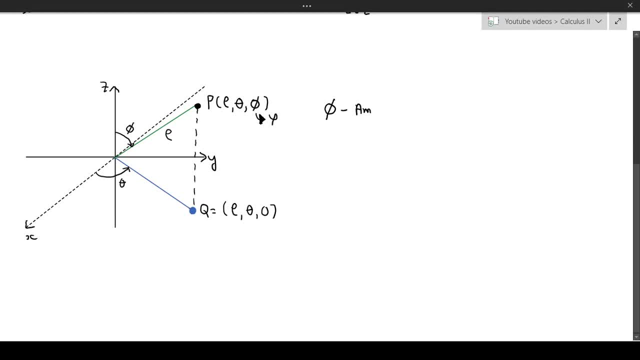 So, in terms of depth, the only kind of range of values you need to consider are the angles from zero, which is right there, to pi, which is at the bottom of the z axis, So the amount of depth. Okay, so that's phi. Now you can think of angle theta as the angle that measures. 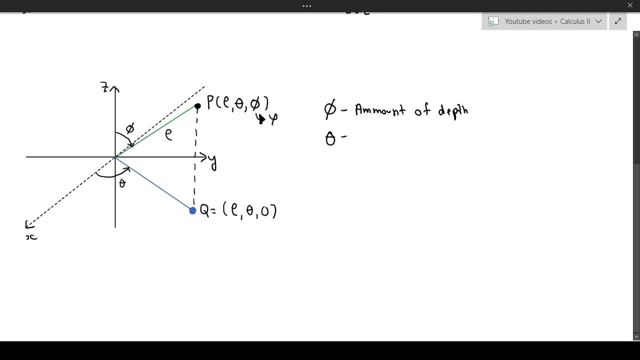 how much in left and right we go in. So you can think of the angle, theta, as the amount that we left and right. That's probably the best way to describe it. So more specifically, it's the angle between the positive z axis or the positive x axis. 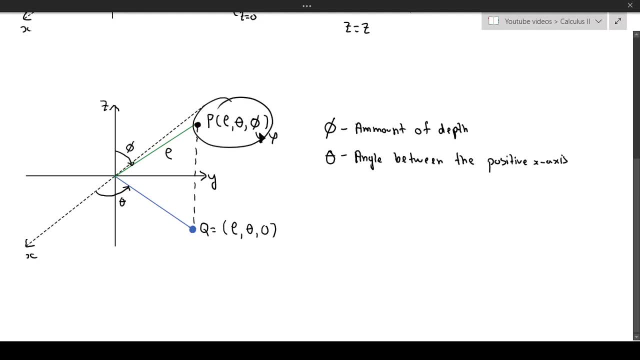 And point q, which is the projection of point p onto the xy plane. So just very cool. Point q is this point projected onto the xy plane. So that's kind of what's going on there: Positive x axis and point q. And just to be very clear, point q is the projection of p onto the xy plane. Okay, 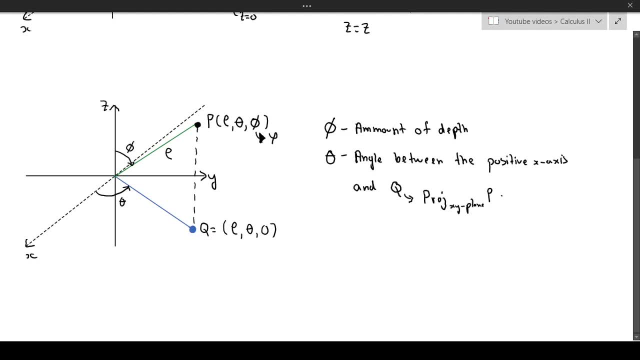 so that's basically angle theta. And then rho is the length of o, which is the origin to point p, So it's the magnitude of that length, So it's magnitude of op, So it's the position vector op, and it's the. 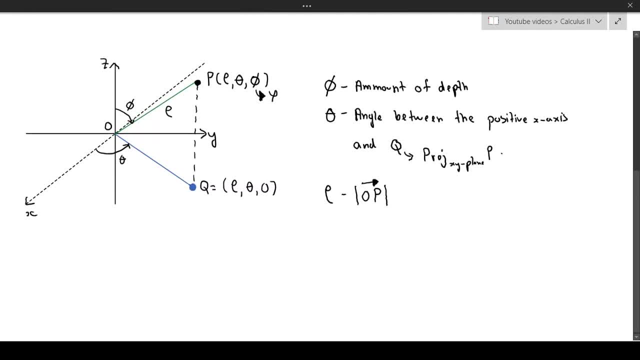 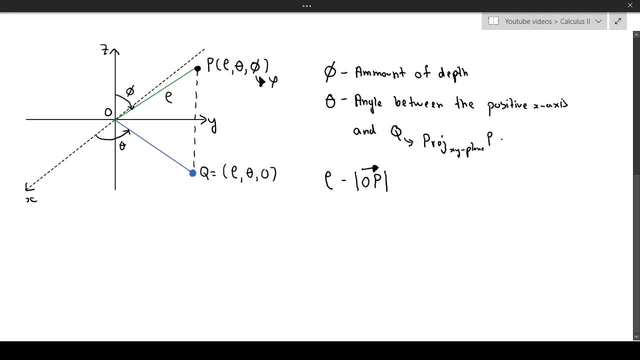 magnitude of that vector. Okay, so that's basically the spherical coordinate system. So let's go and define a few things, as I kind of mentioned earlier. In fact, I'm actually using red because it's actually kind of important, So note: 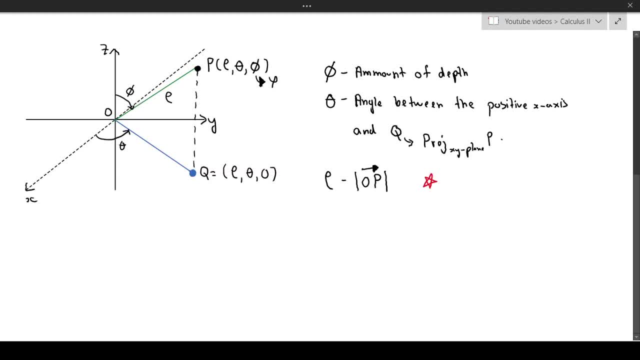 the following kind of restrictions: per se, rho is definitely bigger than or equal to zero, And this is kind of obvious because you know you can have a negative radius or negative length, So that makes sense. Then phi represents the amount of depth in something, So it doesn't. 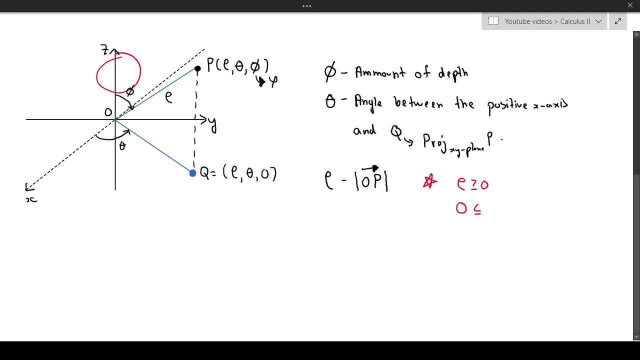 need to go any further than pi. So zero is here and then pi is down here. So I've kind of flipped this around. the angle only goes from zero to pi or zero to 180 degrees. So phi goes from zero to pi And then theta, since it goes from the positive x axis all the way back around. 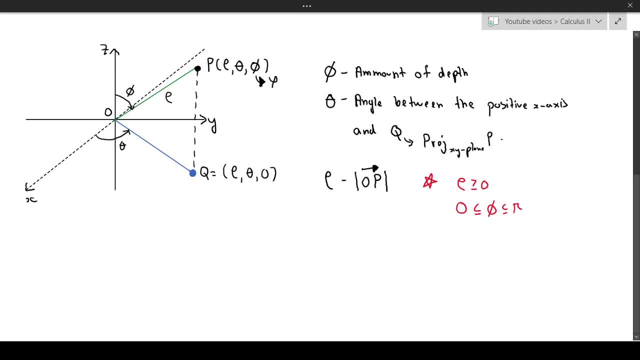 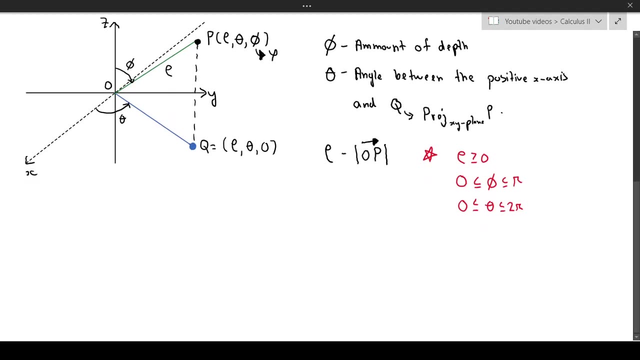 we don't need to go any further than that, because it'll just be redundant. So, obviously, in this case, theta is between zero and two pi, And that will be our well. restrictions for the spherical coordinate system. Okay, how do we actually, you know, convert? 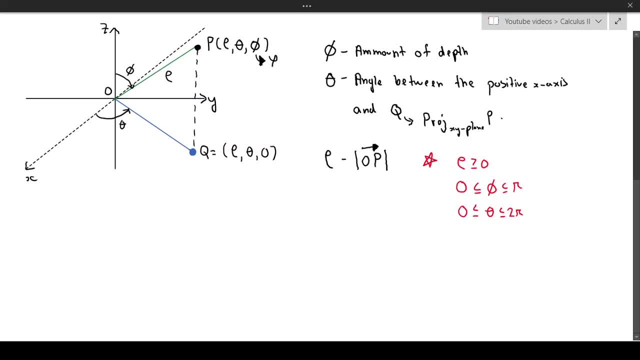 Cartesian to spherical though. Well, let's, let's take a look at that. Well, we can do the following: So x is equal to rho sine theta Or sine phi. sorry, And reason for we're doing this? because rho sine phi. 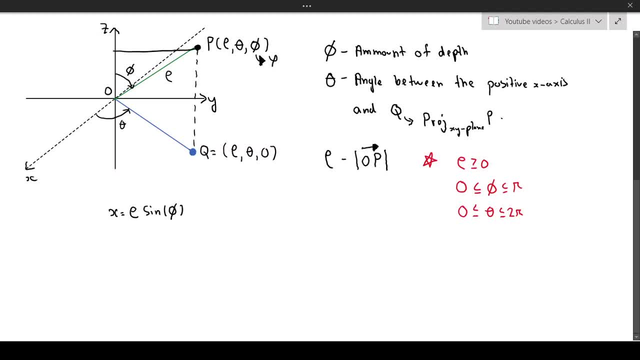 If phi is right there, rho sine phi will give us this length. But this length right there is the same as this blue length. So if you want to project this on to the x axis, well, that's just gonna be multiplied by cosine of theta. So just to be very clear. 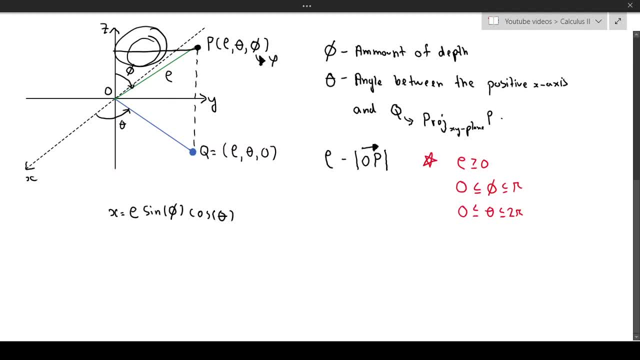 rho sine phi gives us this link right there, But that linked because these are just distance from here here- is exactly the same. This link right there is the exact same as this blue link right there. Okay, and then multiplying by cos, theta will give us this link right there. So this is. 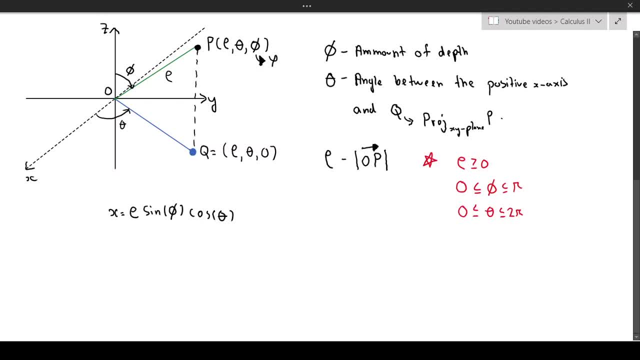 just coming from basic trigonometry. So some basic geometry here, but not too bad overall. Here we we have the same thing with y, but this time we're going to use sine theta, so it's going to be rho sine of phi, sine of theta. And then finally, we have z equals rho cosine of phi. 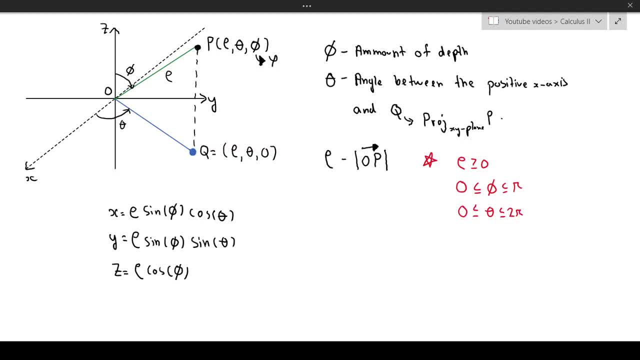 So once again not too bad. And the reason that this works is because once again, if we kind of take the cosine of phi, well that'll just give us this length, but that's exactly the z axis, So that makes sense. So this is the spherical kind of coordinate system. Then 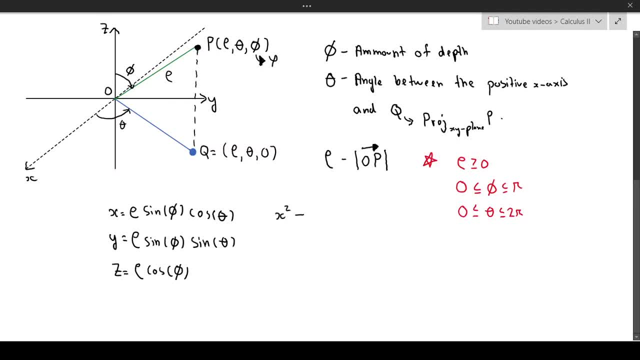 there's one more equation we can use from basic trigonometry, And that is the equation: x squared plus y squared plus z squared is equal to rho squared. So that's another equation that we have to know for spherical coordinates. In fact, I'm actually going to boolean. 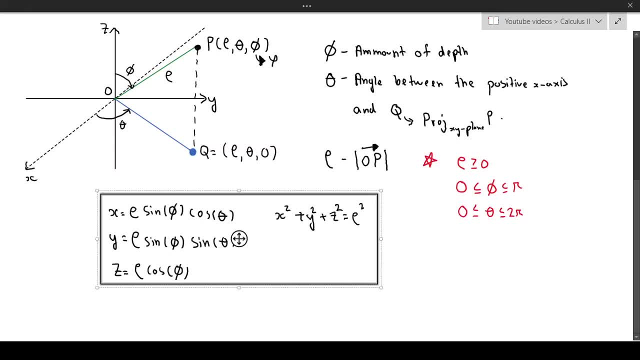 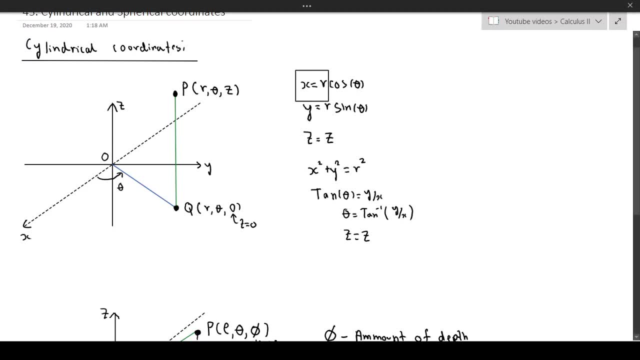 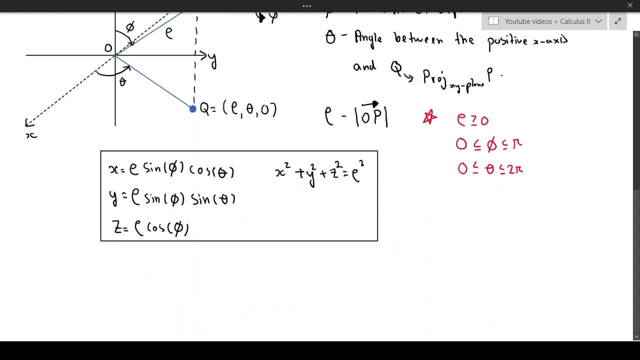 box that, because this is very important, and let's might as well box that box this thing up here as well. so let's go ahead and do that, okay? and with that we have now covered the conversion factors: from cylindrical to cartesian, cartesian to cylindrical, spherical to cartesian, cartesian. 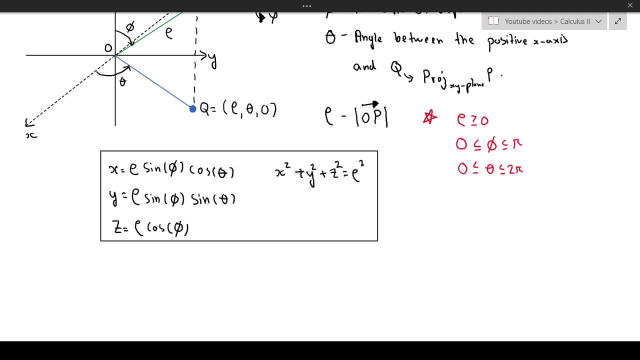 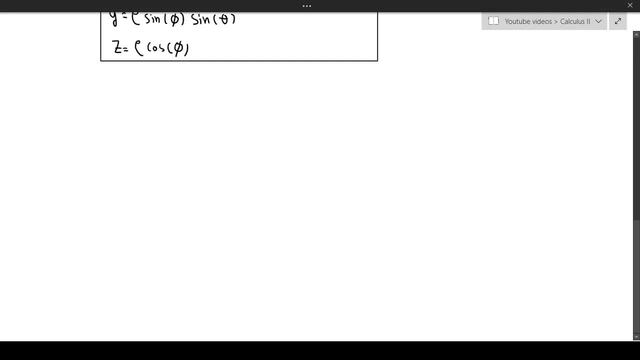 to spherical, so not too bad. okay, now let's do some examples on disk conversion. now some of these examples are going to be very straightforward, but some of these are going to be considerably harder. so let's go ahead and do an example in all these situations. so the first example: 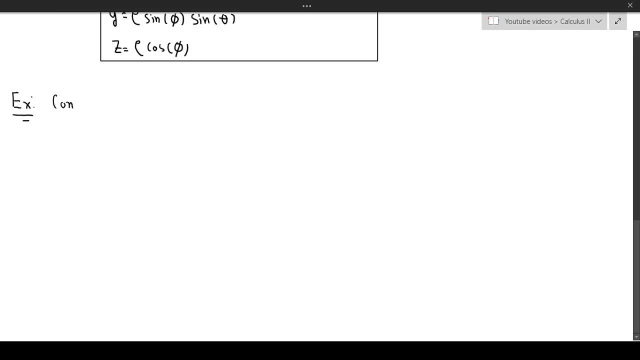 okay, so convert r, theta and z, which is equal to 4 pi over 3 and minus 3 is, into cartesian coordinates. okay, so we can see it's r, theta, z. so we're working with the cylindrical coordinate system here. so here it's going to be: x equals r cosine of theta. then we have y equals r sine of theta. 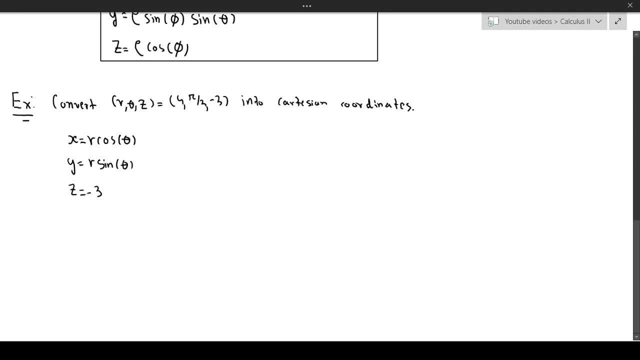 and then z equals to minus 3. okay, so if we kind of write down our conversion factors, well, this is very simple. this is going to be 4 cosine of pi over 3. here we have y equals- that should be a tree, sorry. and then we have y equals 4 sine of pi over 3, and then we have z equals just minus 3. but then 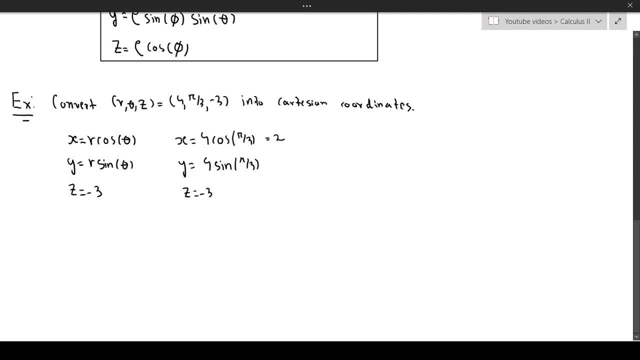 4 cosine pi over 3. if you do it out, you'll just get 2, that's going to be 2 root 3, and that's basically it. so we have finally, in cartesian coordinates we have x, y and z is equal to 2, 2 root 3 and minus 3, so there's nothing special about that. 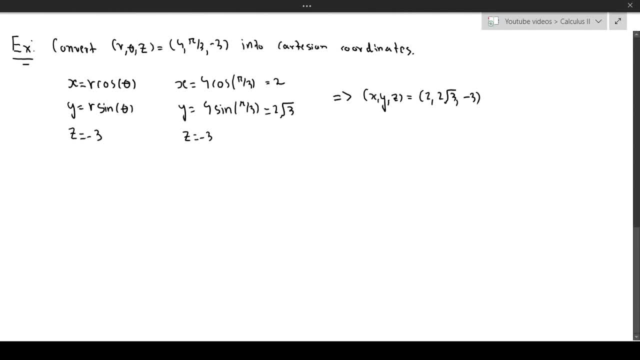 okay, now let's go the other way around. so we're going to convert cartesian coordinates into cylindrical coordinates. so let's figure out how to do that. so let me just copy paste this part and then change the underwording. so: convert x, y and z, which is equal to 2 minus 2 and 1. 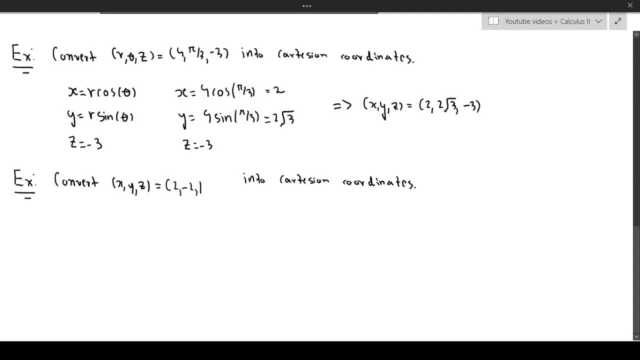 you into cylindrical coordinates. Okay, how do we do that? Well, we can do the following: So we know that x squared plus y squared equals r squared. So x squared plus y squared equals r squared. So it's going to be two squared plus minus two squared is equal to eight. 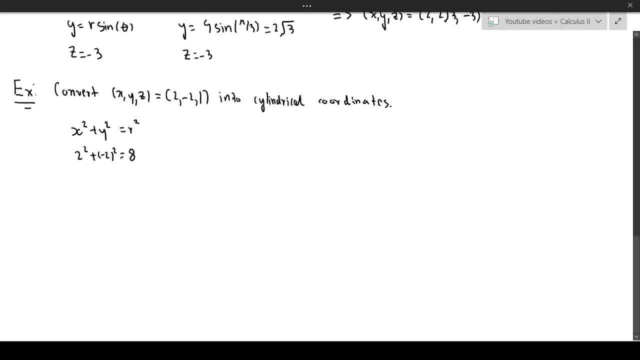 But then we take the square root of this number. So that means r is equal to the square root of eight, or, if you prefer, r equals two root two. Okay, then we know that tan theta is equal to y over x. So theta is equal to tan inverse of minus two over two. 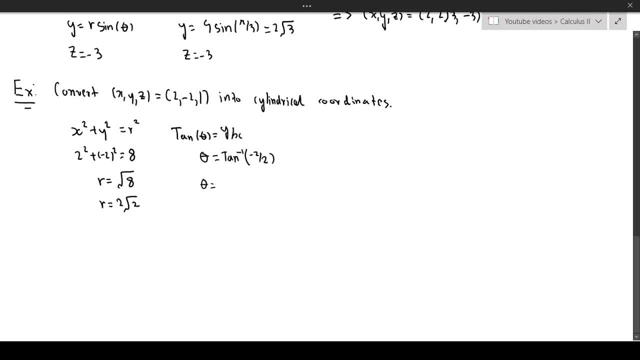 Which is equal to minus pi over four. And the reason it's minus pi over four is because, well, if you take a look at this, we have two and minus two, So it's two in the positive and then in the negative. So we're. 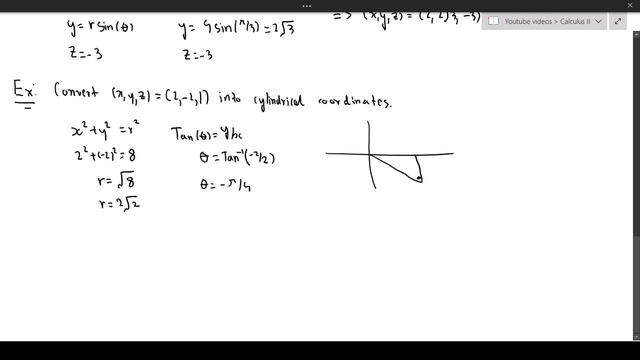 actually in quadrant four. So we have to either subtract the same angle out or we can start a negative of what we have would have had the positive direction. So the angle is going to be minus pi over four, Okay, so just be a little bit careful about that. We have to be in the 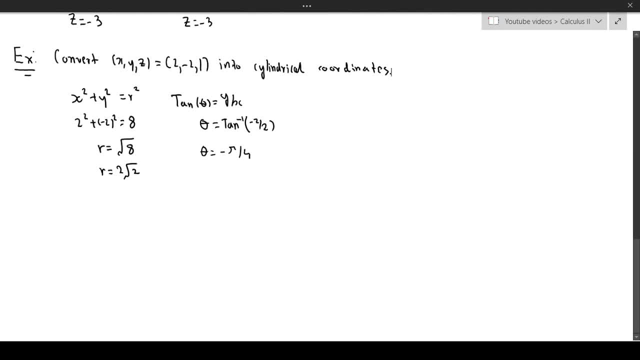 correct quadrant as well. Okay, So we now have theta. So that means r, theta and z are going to be equal, to remember that the z coordinate doesn't change. So it's going to be two root two minus pi over four and one. 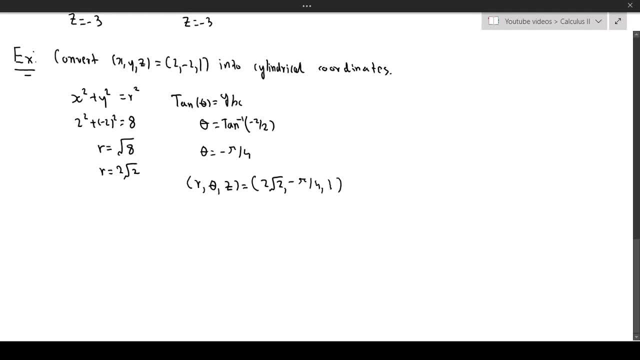 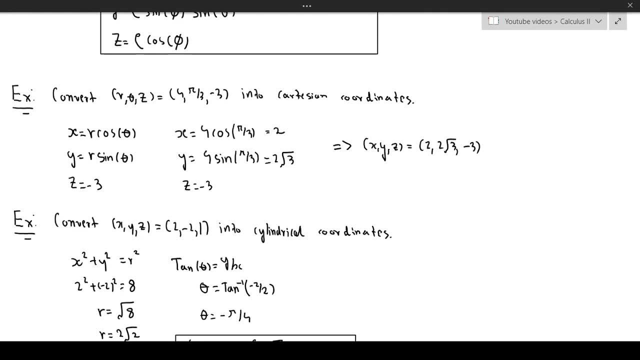 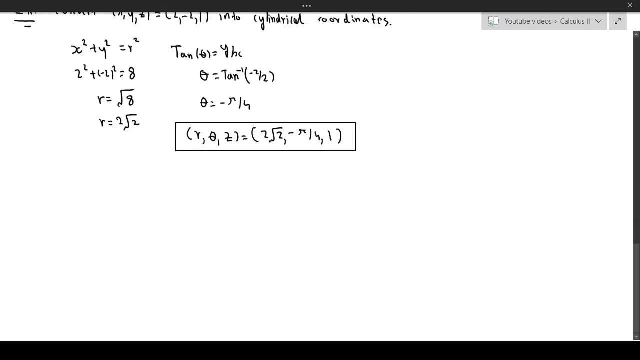 So that is going to be well the answer in cylindrical coordinates. So let's go ahead and box that answer, And let's box this one too, while we're at it. Okay, now let's go ahead and do a very, very quick example. 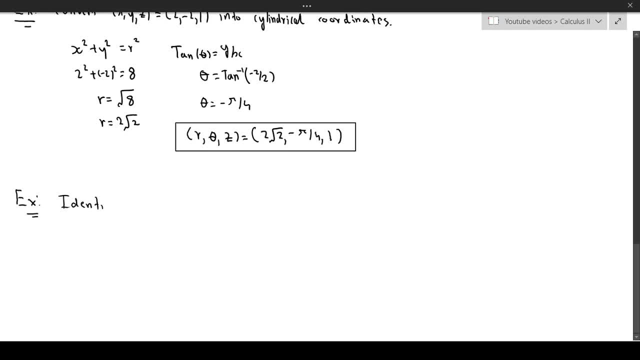 So identify the surface which is given by the equation z equals r squared. Well, this is actually very straightforward. We know that r squared is equal to x squared plus y squared. So we get z equals x squared plus y squared. But then if you, if you go back to my video on the quadric surfaces, we will see that 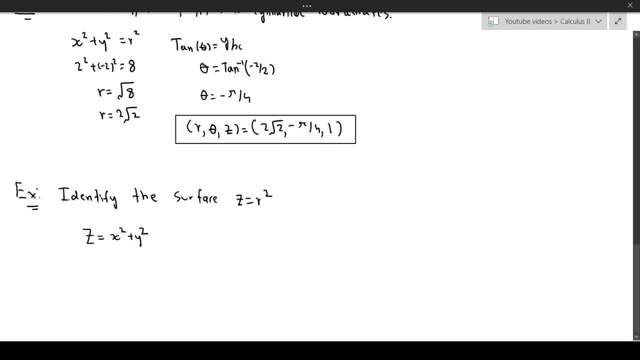 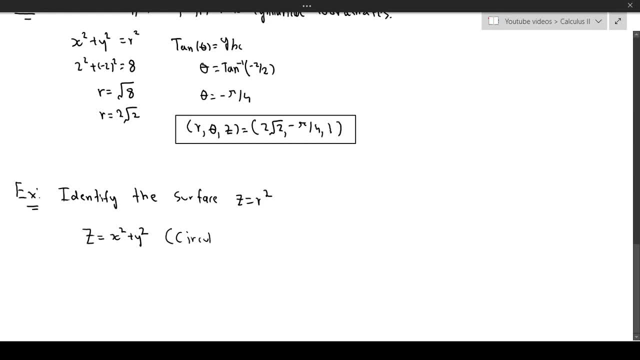 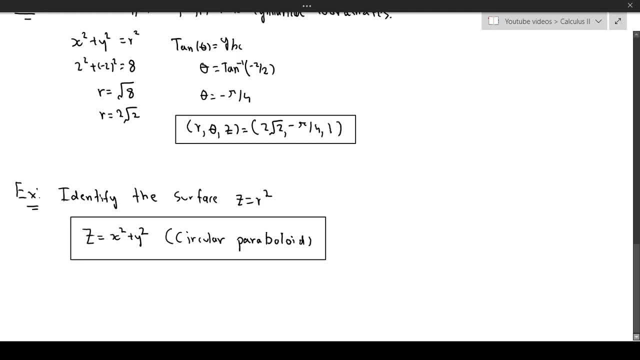 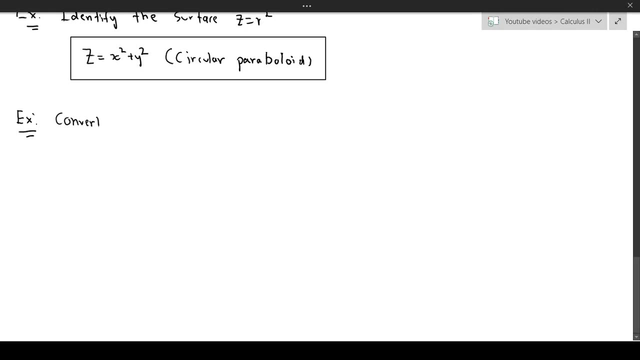 about this. we just have to be able to identify certain surfaces by conversions. Okay, let's do more examples. So this time we're done with cylindrical coordinates, So we're going to be doing examples with spherical coordinates now. So convert x, y, z. 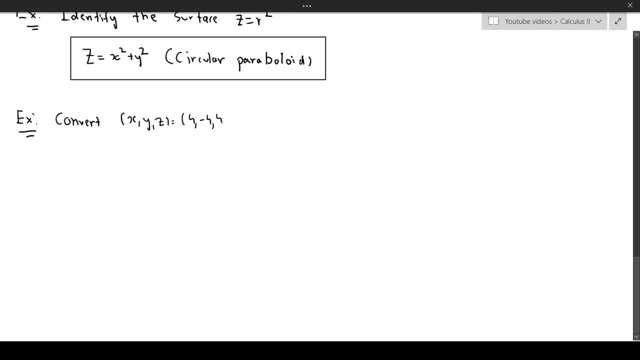 which is equal to four negative four and four root six into spherical coordinates, or spherical coordinates, depending on how you pronounce it. Okay, how do we do this? Well, we know that rho is equal to the square root of x squared plus y squared plus z squared. And we know that because 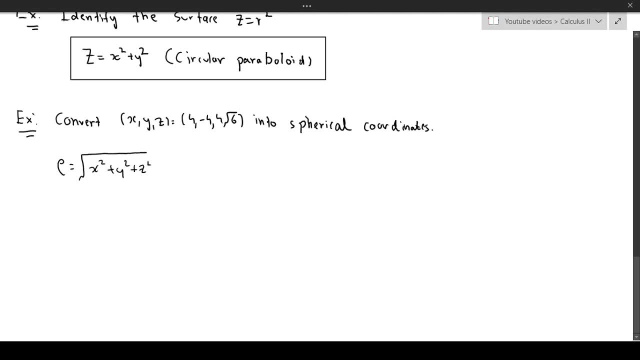 rho squared is equal to x squared plus y squared, plus z squared. So that means rho is equal to the square root of four squared. so that's 16, plus negative four squared, that's also 16.. And then four root six squared, that's equal to 96.. Okay, but then rho is equal to the square root. 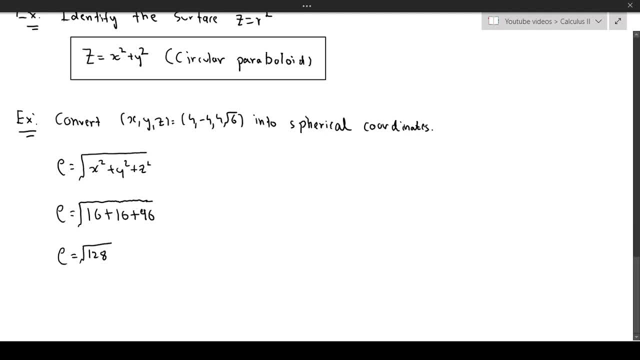 of 128. But then this is equal to eight for two. Okay, so, once again, not too bad. So we now have rho. Remember we also need theta and phi. Well, theta is not too bad, we know that, tan theta. 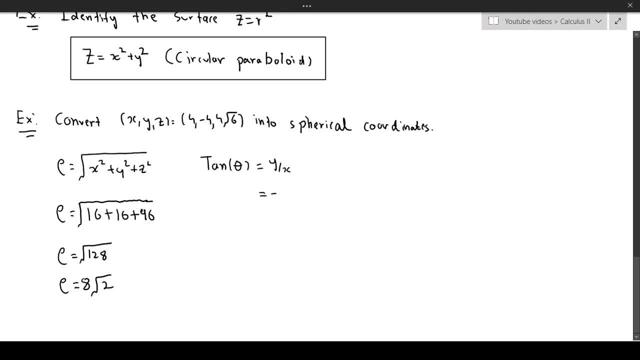 is equal to y over x. So we know that is equal to minus four over four. So theta is equal to tan inverse of minus one. So we could once again write minus phi over four. But let's just, you know, write this in terms of positive coordinates, because why not? So once again, just be really. 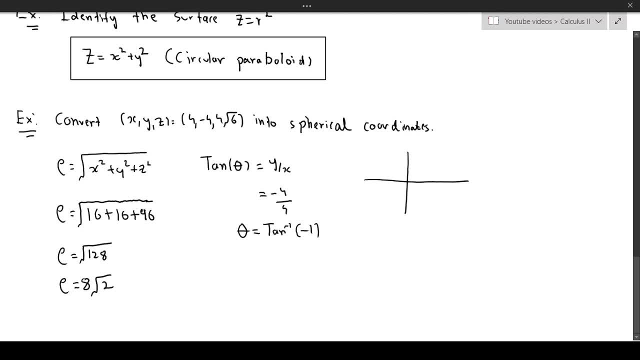 clear Negative four and four implies that we have the positive x axis is four, because it's positive x and then negative four is to y direction, meaning that our angle is right there. So we can't- you, we could, we, could I- raise minus pi over four, or we just go all the way around and 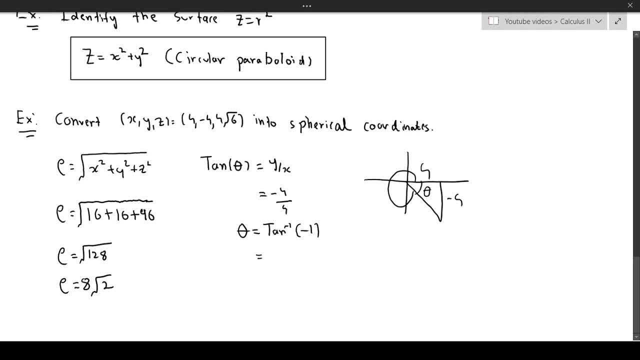 get the positive angle. So we have zero four plus T, plus negative four plus x, and then negative four more, because we can get the positive x And we have negative four. god, so I don't have. we could also say this is equivalent to writing seven pi over four, So that's the exact same. 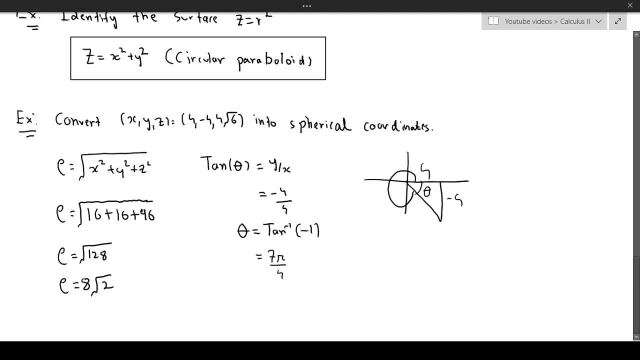 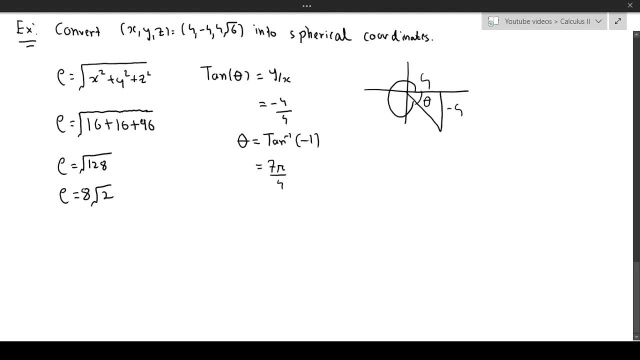 thing. So there's nothing special about this, Okay. And next we can kind of get. we can figure out what phi is equal to. So we know that rho cosine of phi is equal to z, So that means we get eight root two. cosine of phi is equal to four root six, Meaning that by definition, 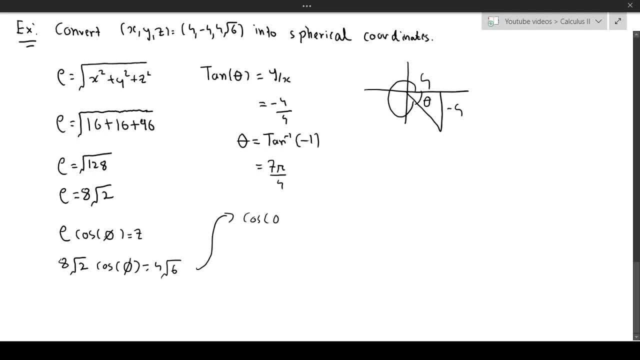 we have, cosine of phi is equal to root three over two and that just comes from dividing. So that means phi is equal to cosine inverse of root three over two. But then this is equal to pi over six. And remember that by definition we need to ensure 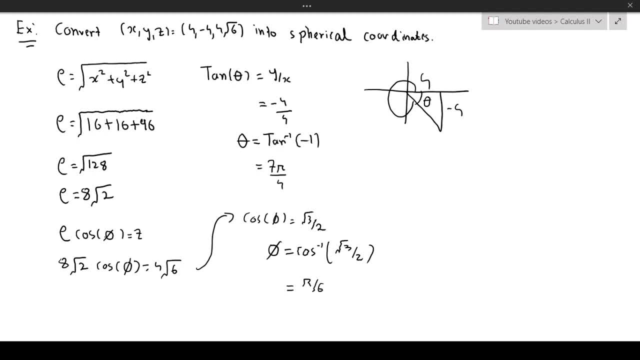 that phi is between zero and pi, But pi over six is an angle that's between zero and pi, So there's nothing wrong with that And we are good to go. So that is phi. So, as a result, we get the following situation: we get rho. 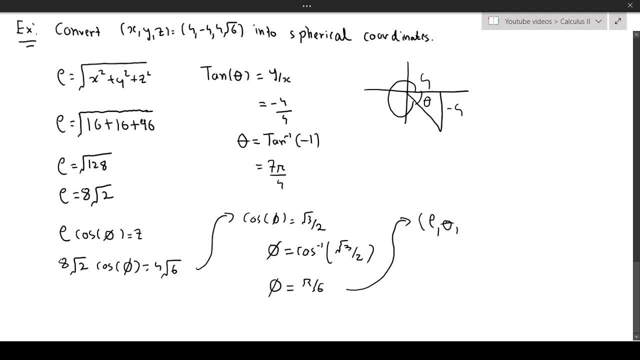 theta and phi is equal to eight, root two, seven, pi over four and pi over six. And that, right, there is our angle. So let's go ahead and just box that answer And we're good to go. So that, right, there is our conclusion. So that, right, there is our conclusion. 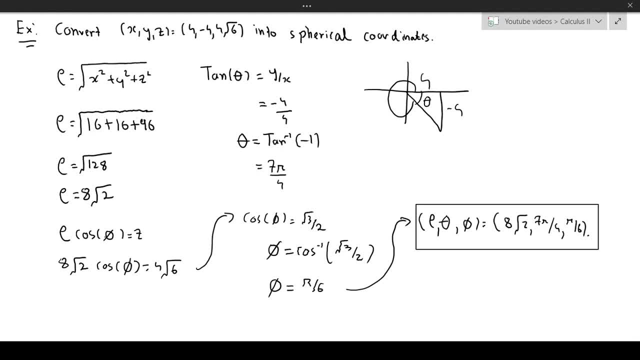 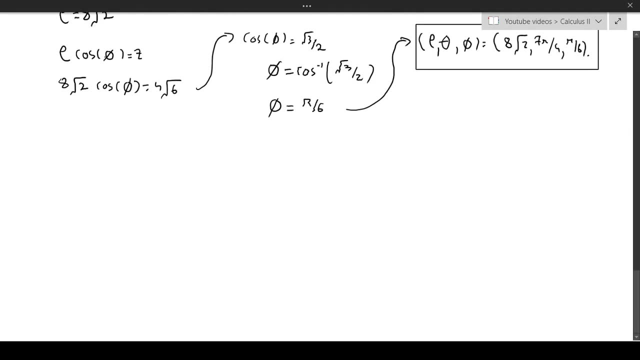 Take some of that example. So let's do another example. So we have a few examples in this part. Okay, so we have about three more, four more examples to go. So there's a lot of examples here, But I think this will cover just about everything you can be asked in terms of spherical 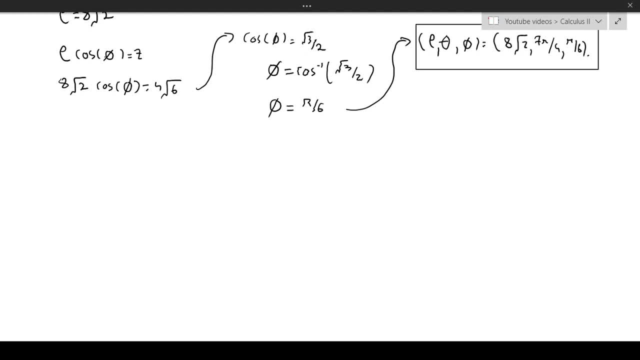 coordinates for a standard calculus two course. So let's go ahead and do this example. So this time I'm going the other way around. I'm converting from spherical into Cartesian. Let's go ahead and do this example. So this time I'm going the other way around. I'm converting from spherical into Cartesian. 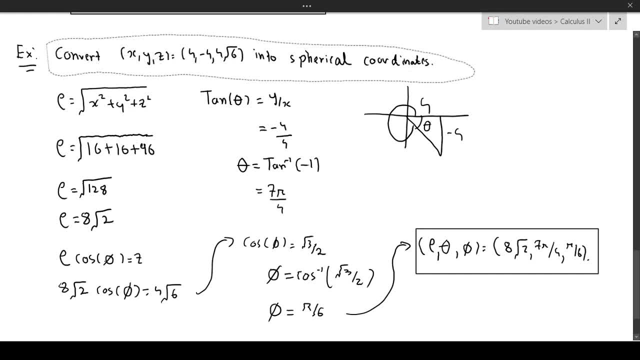 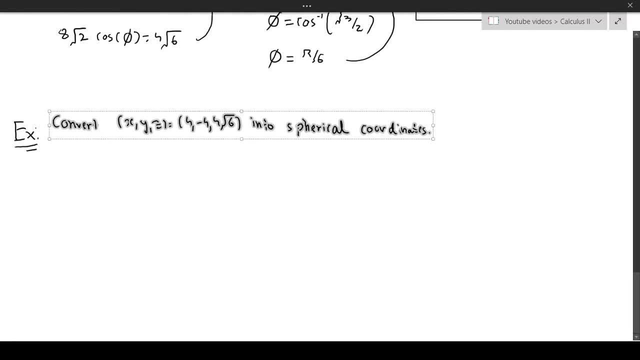 Luckily, this is much easier, So this one required you to do some grunt work, But converting from spherical to Cartesian is very simple. we would quite literally just plug it in. So this copy is that same thing, because it's going to be almost the same thing. So this time, 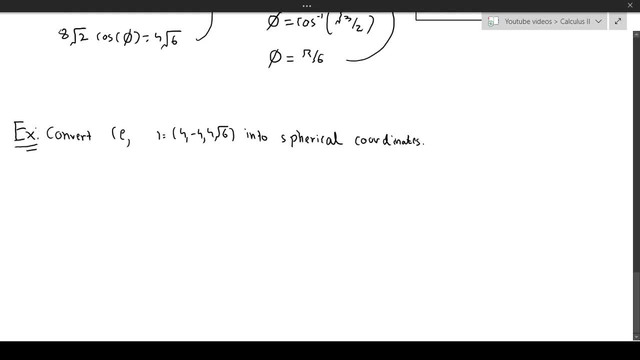 it's going to be rho, theta and phi, And this one is going to be four: pi over three and pi over four. Okay, but this time we're going to go in converging this into rectangular coordinates or Cartesian coordinates. 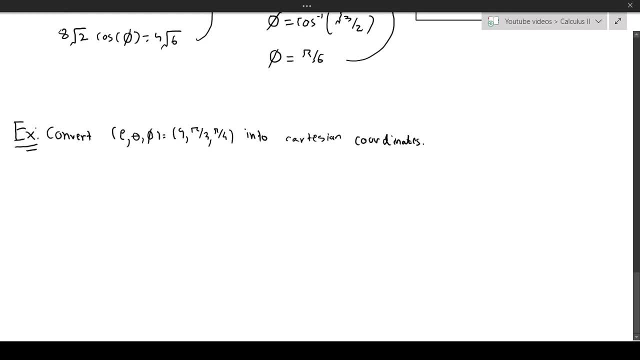 Okay, so we can proceed with this example the same way we did it in terms of the normal Minors coordinate system. like we. in terms of like, converting from cylindrical to Cartesian, except equations masala blade, a different differentかすか we и Uh-иши. 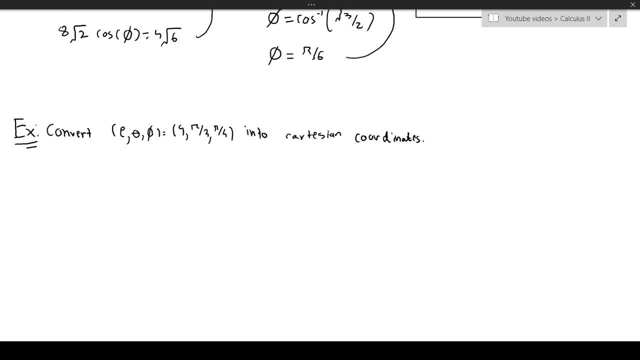 eg عند, eg 할�, dumpling eternal. a little bit differently. These expressions are гомний冷원ESf. alright, a little bit different this time. So in this case we have the following: So we have x is equal to rho sine of phi, cosine of theta. We have y is equal to rho sine of phi sine. 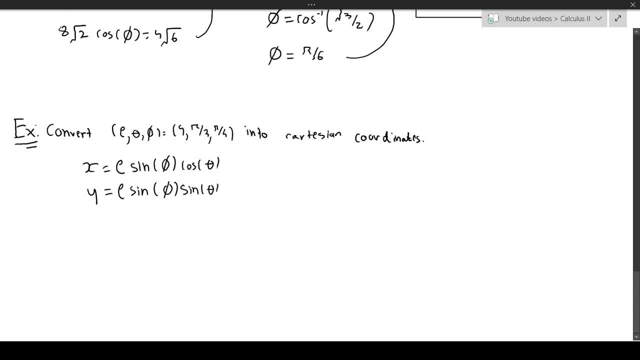 of theta. And finally we have: z is equal to rho, cosine of phi. Okay, so let's go ahead and convert these coordinates over, So this means that we end up getting x is equal to rho, so it's going to be four sine of phi, which is going to be pi over four. 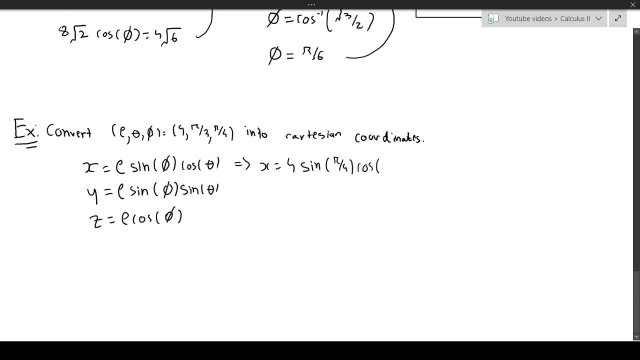 And then cosine of pi over three, But then this itself is equal to root two. Okay, so now we have y equals four sine of pi over four, And then cosine of- or sorry, not cosine sine of- theta, So that's gonna be pi over three. If you go in and write that out, you'll get root six. 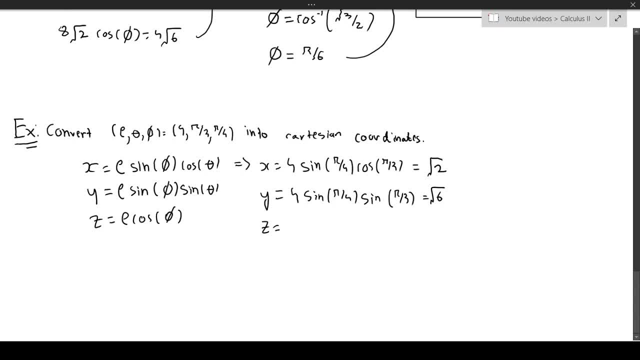 Then, finally, z is equal to rho. cosine of theta, so it's going to be four. cosine of phi- sorry, so it's gonna be cosine of pi over four is equal to two root two. Okay, so that means, in terms of the coordinate system, the Cartesian coordinate system you have. 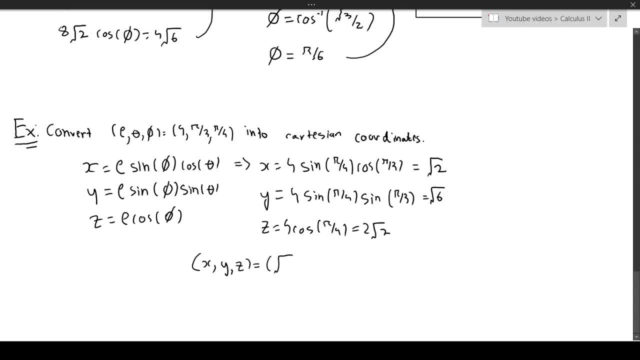 x, y and z is equal to root two, root six and two root two. And that, right, there is going to be our conversion coordinates. All done, So let's go ahead and move this over, And that, right, there is going to be our answer. So we're done. Okay, now we can also convert. 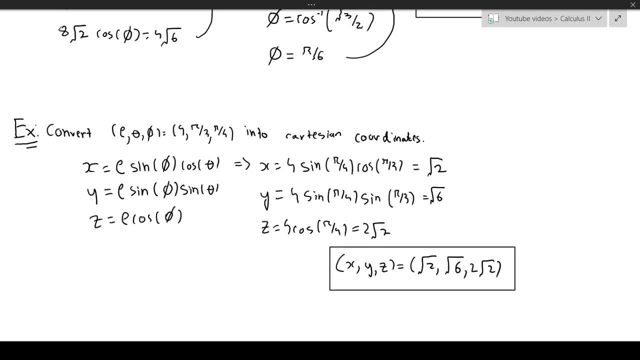 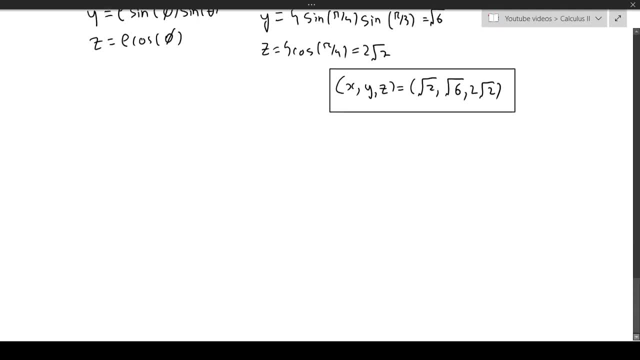 a lot of equations as well. So let's do an example of converting equations into, well, spherical coordinates and cylindrical coordinates, as necessary, but we will be mostly working at spherical coordinates here. So let's go ahead and convert this equation. So example, So 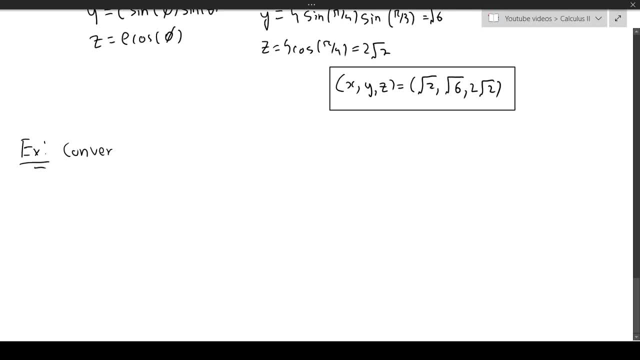 convert z equals- z equals the square root of x squared plus y squared, into spherical coordinates, or spherical coordinates Okay. So let's go ahead and do that. This one isn't so bad. So we know that z equals rho. cosine of phi. 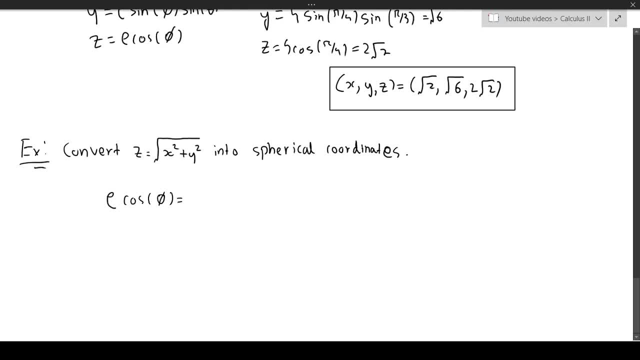 And then here- well, let's be a little bit careful here. So if we go ahead and put the square root here, we'll get x equals rho sine phi, cos theta all squared. So we end up getting rho squared sine squared of phi, cosine squared of theta. And then here we get. 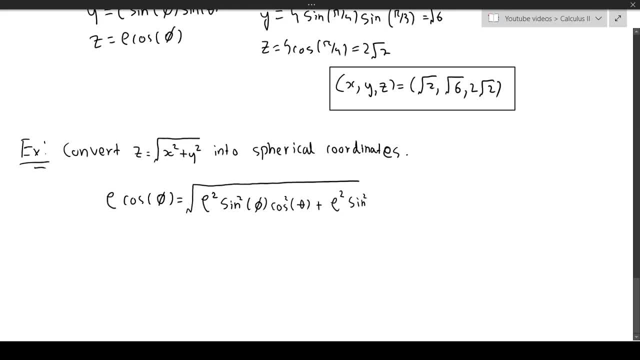 rho squared sine squared of phi, sine squared of theta. Okay, So now we can factor the rho sine squared out, so we can factor the rho squared sine squared And then, if you go ahead and do that, we are left with rho sine of phi, And then we have the square root of sine. 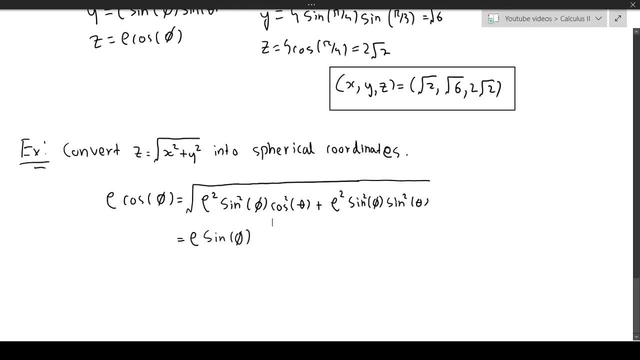 plus cos squared, but we know that's equal to 1, so we can just write 1 instead. so we get rho sine of phi and then if you go ahead and divide both sides, so just to be very clear, this is rho cosine of phi and then rho cosine of phi. but then if you go ahead, 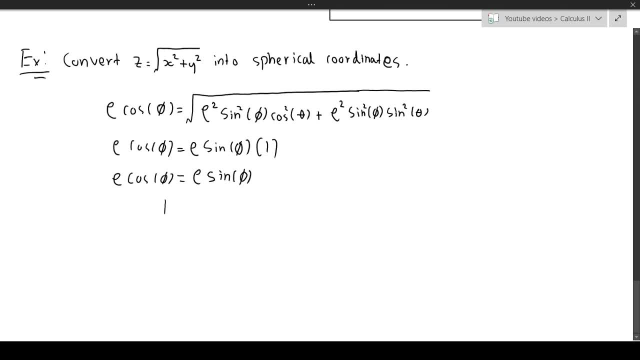 and divide this, we'll get: 1 is equal to tan of phi, but then phi in this case we're assuming positive orientation, so we get pi over 4, so just to be very clear, if you look at the chart for coordinate surfaces, this is a cone. so in terms of spherical coordinates, 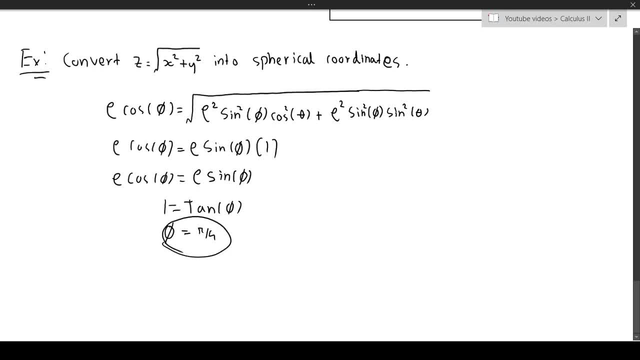 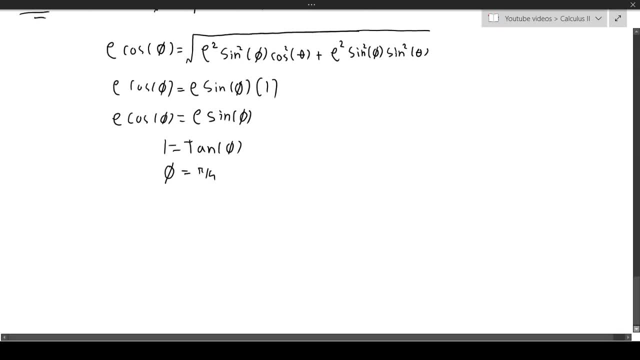 the cone can just be represented by an angle, so that's very nice. Okay, let's do an example of writing a description of a solid in terms of spherical coordinates. so what do I mean by that? So let's go ahead and do this example. Okay, so a solid lies. 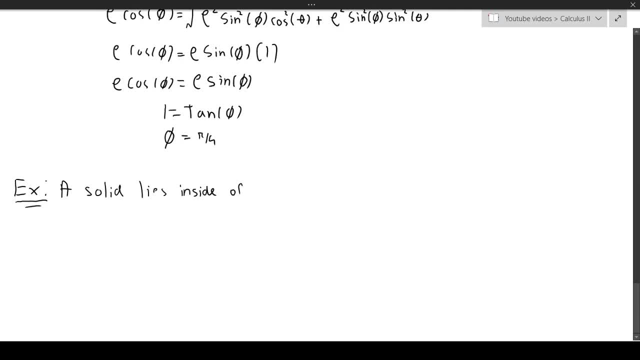 inside. Okay, so a solid lies inside. Okay, so a solid lies inside of these surfaces. x squared plus y squared plus z squared is equal to 1, and z equals the square root of 3 times x squared plus y squared. Okay, just to be very clear, this: 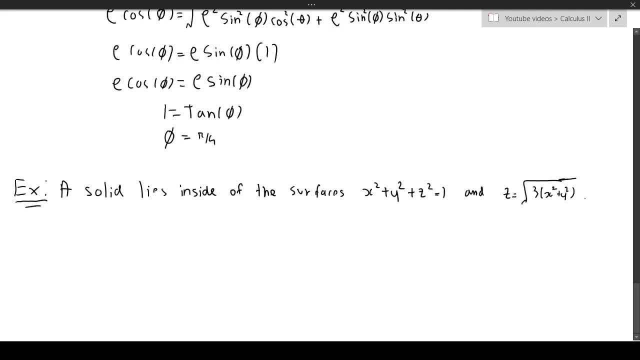 is a solid. Okay, now let's take a look at this actual example. So write a description of the solid in terms of inequalities of these surfaces involving spherical coordinates. Okay, so how do we use inequalities to describe this? Well, we can do the following. Let's actually just convert these surfaces straight. 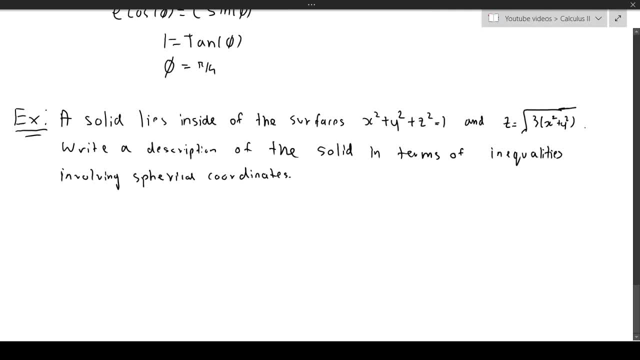 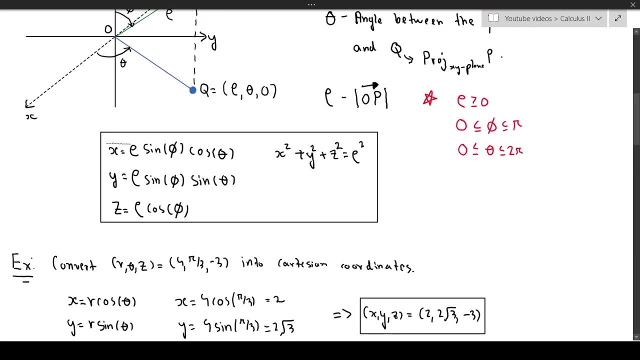 up into spherical coordinates. So, to be very clear, let's just copy down these surfaces and we're going to just run our conversion formulas, which I'm just going to do from here, So that way we have a reference to what we actually use to improve the conversions. 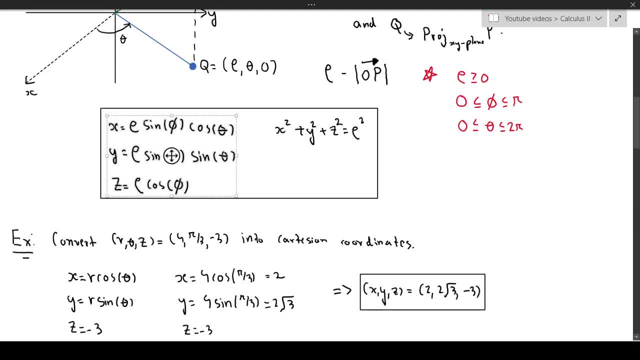 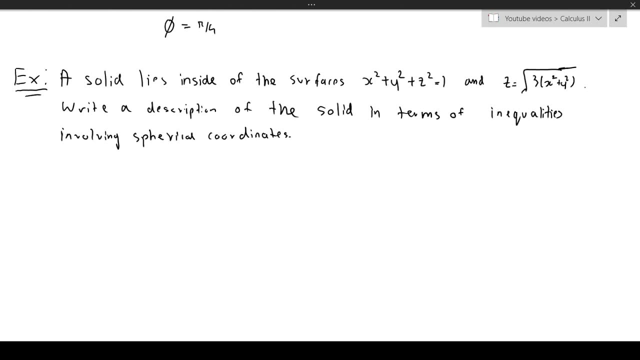 So I'll just go ahead and do that really quickly. In fact, I can just use the whole box actually, because we need all four of these, Okay. Okay, so this is our coefficient. Okay, so we can use the equation of the sphere and the cone here. so let me just put those. 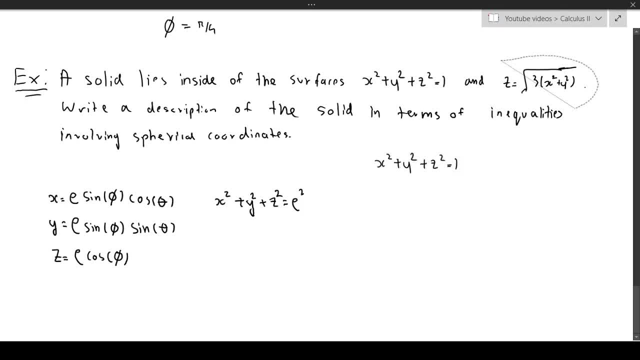 down as well here. Okay, so right away from this equation, we can get rho. so we know that x plus y square plus z square equals 1, but that's equal to rho squared. so that means rho equals 1, and we don't assume that rho is positive, if you remember, because the link 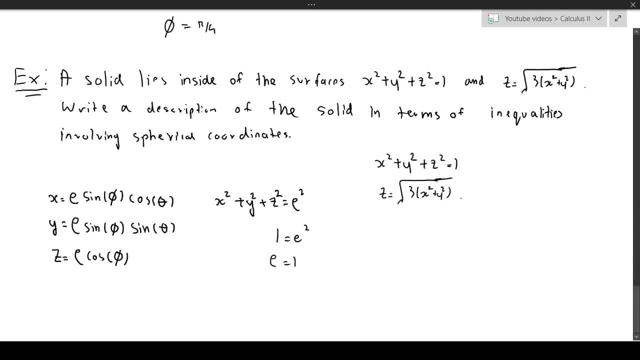 cannot be negative. so that means, by definition, rho is equal to 1.. Cool, so we always have to use the equation of the sphere and the cone here. so let me just put those down. and we already have a description for one of these things. Okay, we also are not. 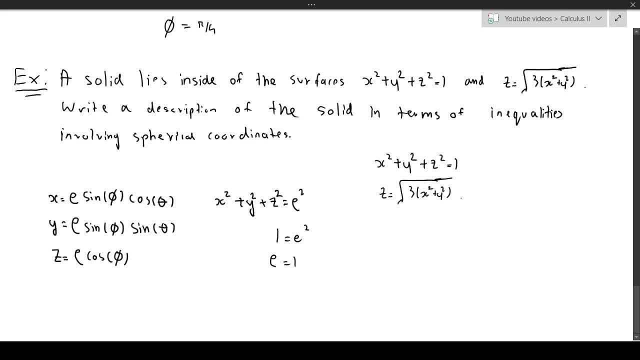 restricting the equation of the sphere in any way. we haven't restricted the range of values for theta. it's still a sphere. we haven't restricted it in any way. so we automatically know that for rho, rho is between 0 and 1, and then we also know that for theta, theta. 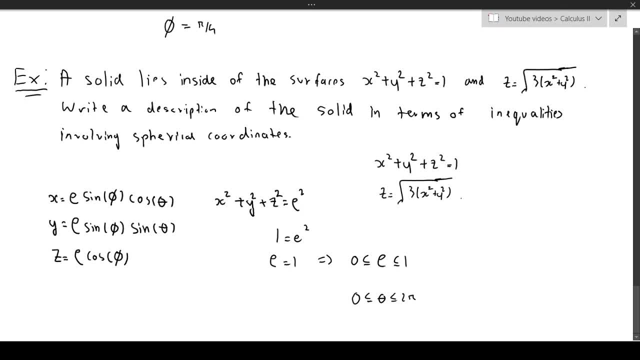 is between 0 and 2 pi. We just have to figure out what phi is. so- and let's just be very clear- I'm going to write phi using this angle. We could have also used this, but it doesn't really matter. 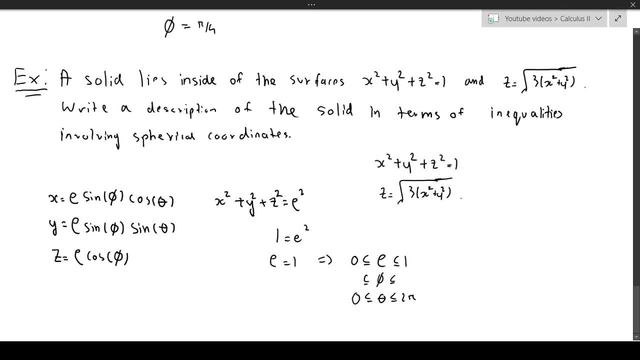 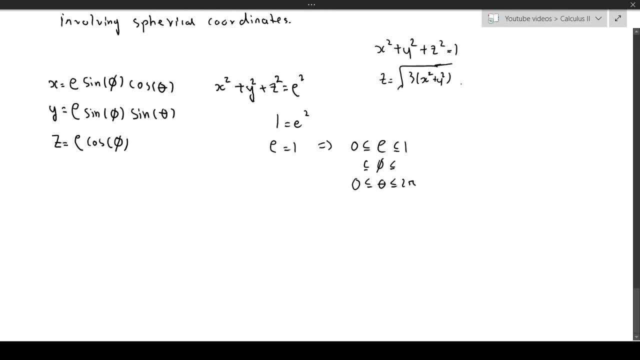 that's also phi. it's just a matter of choice. So we need to figure out what phi is. Well, there's no obvious way to get that, but what we can do is use the cone and then hope something nice happens. So let's go ahead and do this out. So z equals rho. 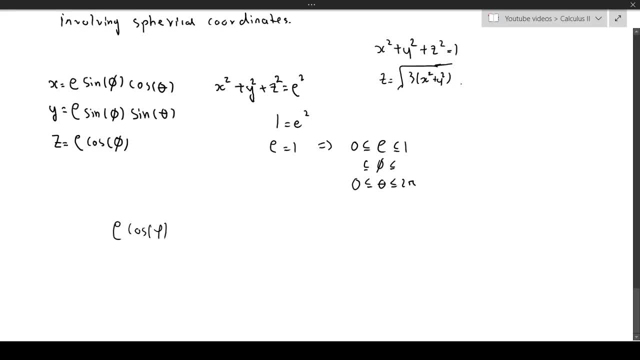 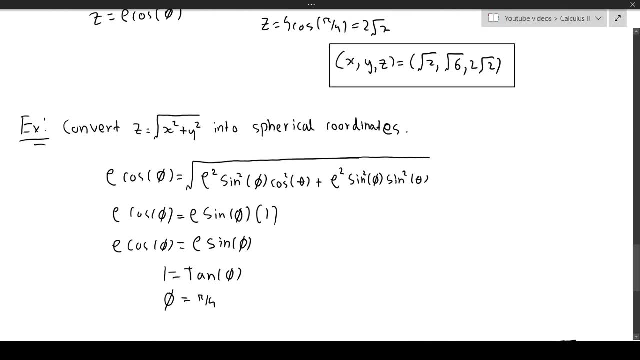 cosine of phi. we'll just kind of use this here as well. it doesn't really matter. Now let's go back up a little bit. We actually used this just a moment ago here. This part right there was just equal to 1, and then just pulled the rho sine phi out. So we actually 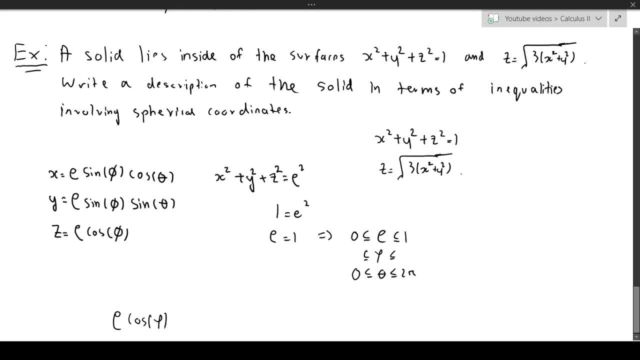 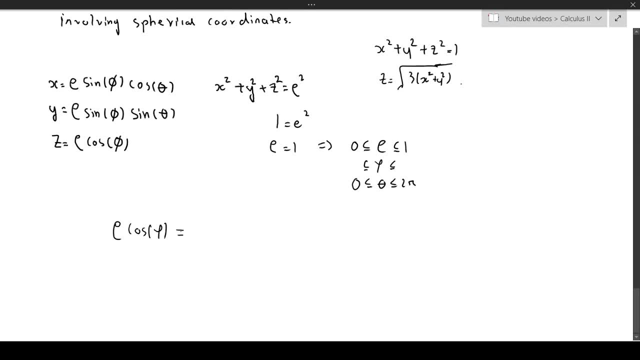 did most of this already. So as a result, the only difference here is that we have root 3.. So we should get a similar kind of result when we do this out, just as a sanity check of sorts. So let's go ahead and actually do this out. So if you convert these coordinates, you'll 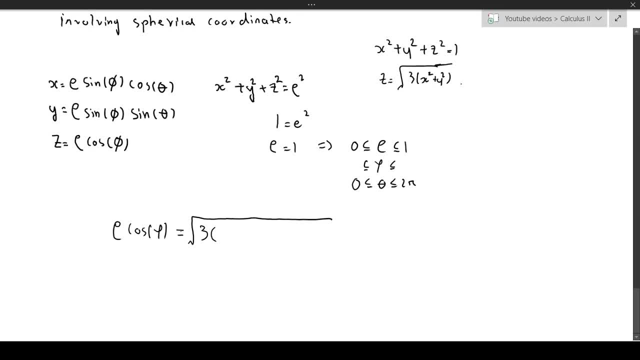 get 3 times x squared plus y squared. so it's going to be just to be really clear: if you distribute the 3 out, we'll get rho squared sine squared of phi, cosine squared of theta, plus 3 rho squared sine squared of phi. 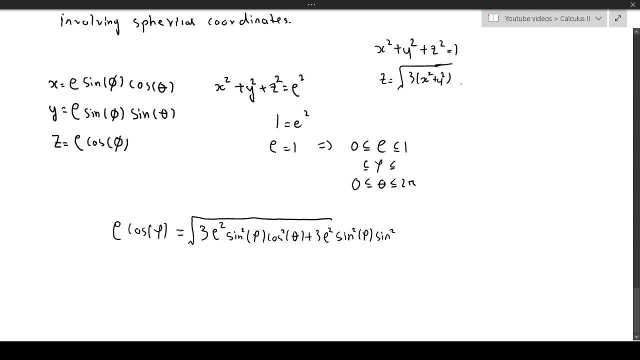 sine squared of theta. Okay, so what can we do now? Well, one thing we can do is we can pull the 3,, which is common to both of these terms. We can pull the rho squared, which is common to both of these terms, and we can also pull the sine squared phi, which 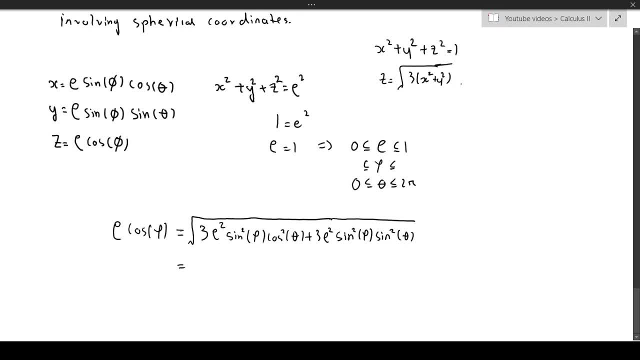 is common to both of these terms. So overall we're going to end up with root 3, rho sine of phi, and then we're left with cos squared plus sine squared. but that's just 1, the square root of 1. 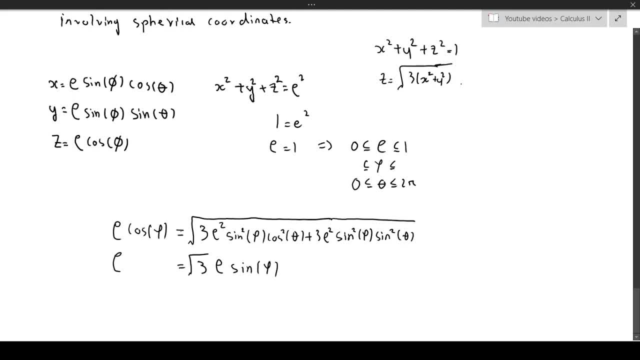 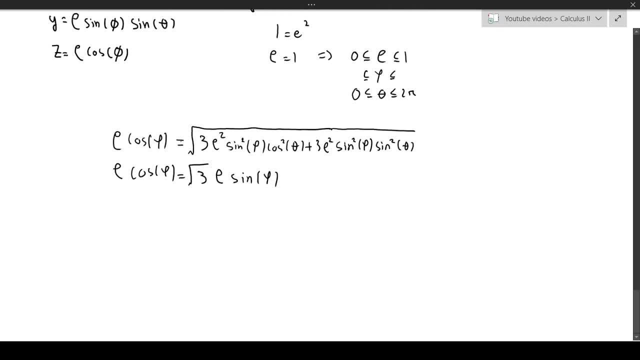 is 1, so we're done there, and here we get rho, cosine of phi. Okay, so now we end up with 1 over the square root of 3 equals can of phi. so phi, if you go ahead and find this angle. 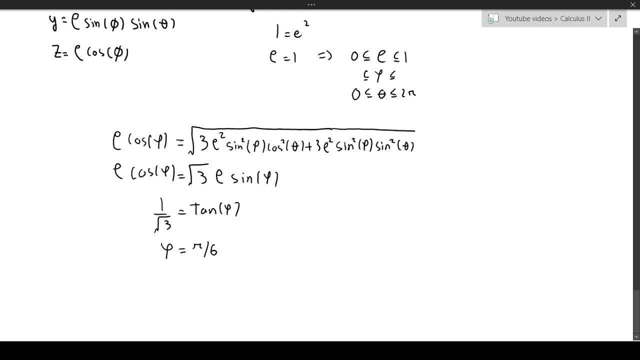 is equal to pi over 6, and that, right, there is our answer. so we get that 0 is less than or equal to phi, which is less than or equal to pi over 6, and that, right there is our description of this. 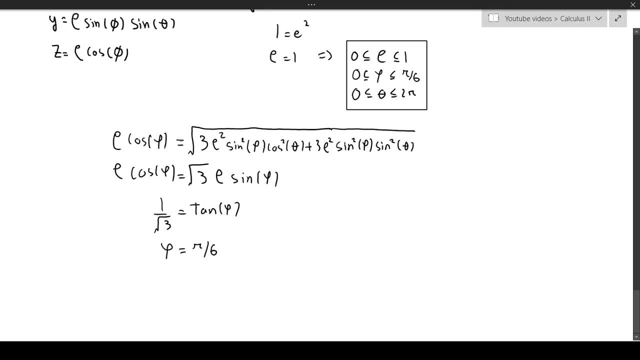 particular solid in terms of inequalities. so if you're wondering what this looks like, it's the positive half of a cone, because it's the positive square root. so here's the cone, and then we kind of have this little half sphere intersecting it. 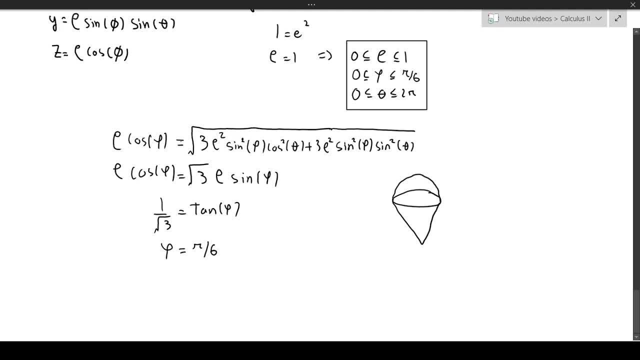 so it kind of looks like this. so it basically looks like an ice cream cone of sorts, for lack of bad words. so that's what the solid will actually look like if you draw it out. but, that being said, you don't need to draw a solid, so we're done with the example. 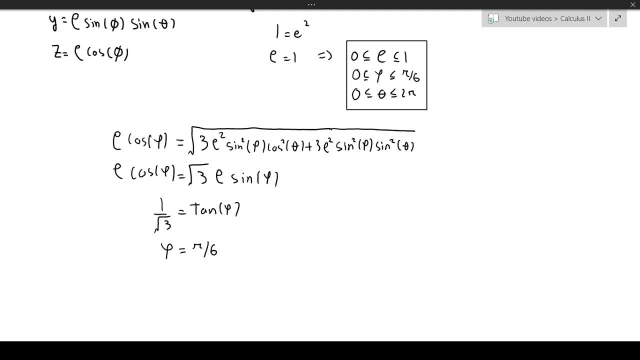 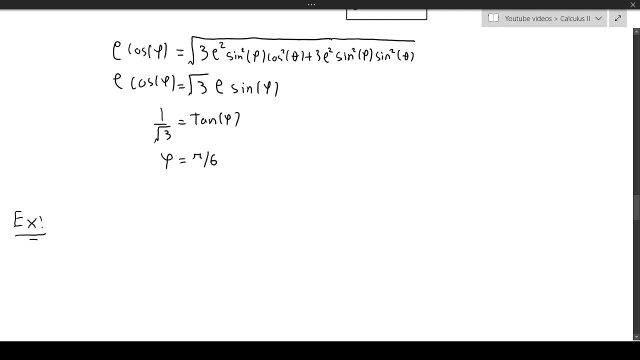 Okay, let's do one more example, and that'll be it for this video. Okay, so this one is a bit of a long question, so bear with me while I write this down. Okay, so find an equation for the surface. 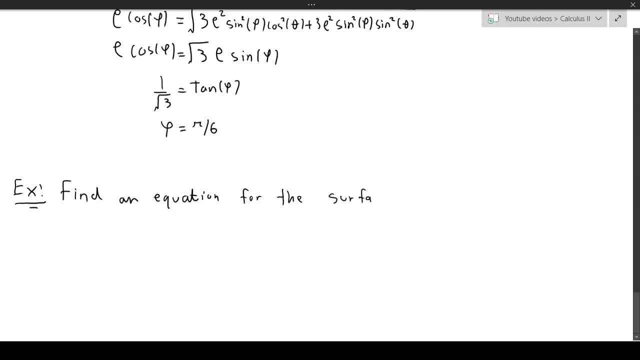 consisting of all points which we could denote as x, y and z that are three times as far from the point zero, zero and nine as they are from the plane. z equals one, Okay, Okay, Let's go ahead and write this down. 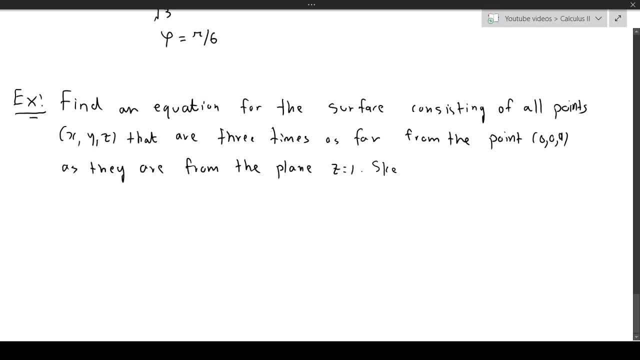 The rest of the question. so sketch- let's try and remove the word sketch. we don't need to draw, we're not going to draw this part, so, yeah, sure, let's just draw it anyway. so sketch and identify. and. 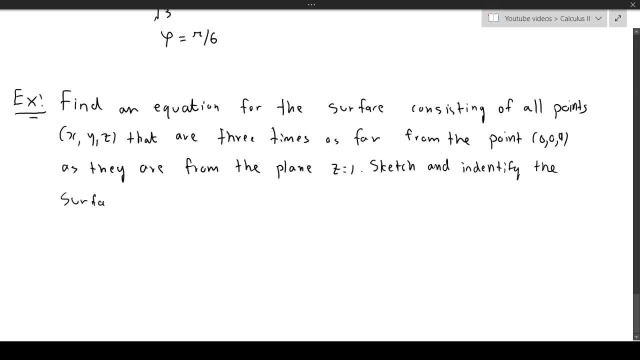 the surface. Okay, and then write an equation in spherical coordinates or spherical coordinates for the obtained surface. Okay, i'm going to have some alphanSwitch So I just want to write it out. so guess it's two, is it two ones? 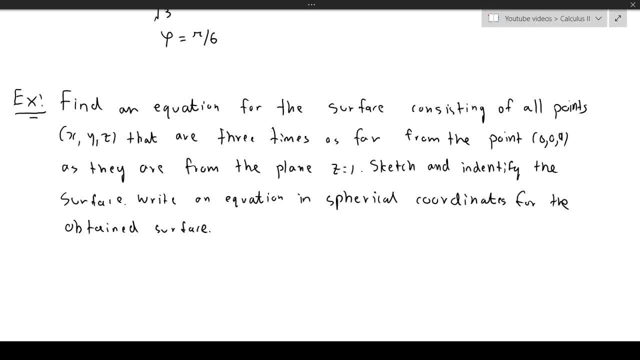 Yeah, yeah, yeah, okay. Oh well, my at this point, that's it for this one. It's very effective. we also have to convert this into spherical coordinates at the end. So how do we even begin to comprehend this question? Okay, so one of the easiest ways to kind of start this question off: 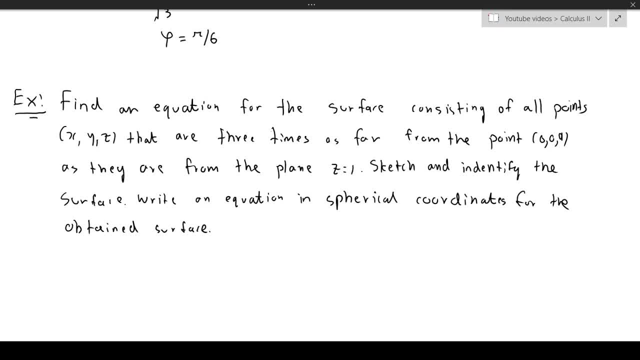 is to kind of take a look at this. We're told that the distance from the point to the point is three times the distance from the point to the plane. Okay, so that just means that, by definition, we can use the distance formula to find the distance from the point to the point. 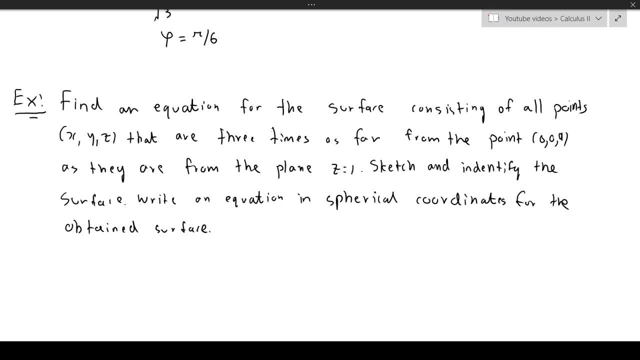 and we can use that formula that we kind of derived a few or we talked about a few videos ago, to find the distance between the point and the plane. And then, since we're told the distance from the point to the plane is three times as far, we just multiply the distance from the point. 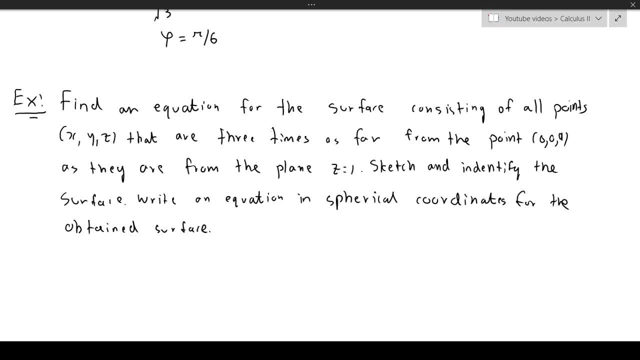 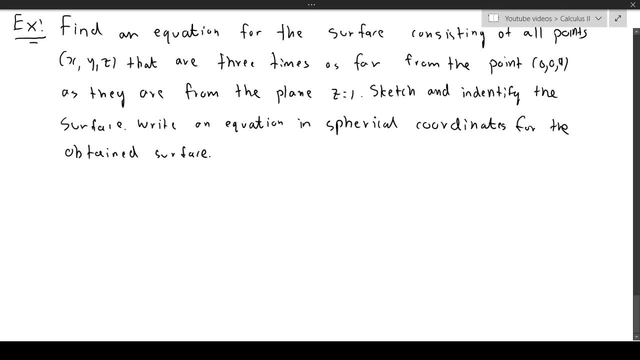 to the plane by three and get a relation that way. Okay, so how do we actually, you know, do that? So this is probably easier to set this up. So let some point be denoted by the following. So I'm going to call this point x, y and z. Okay, so let's keep going. So the plane. 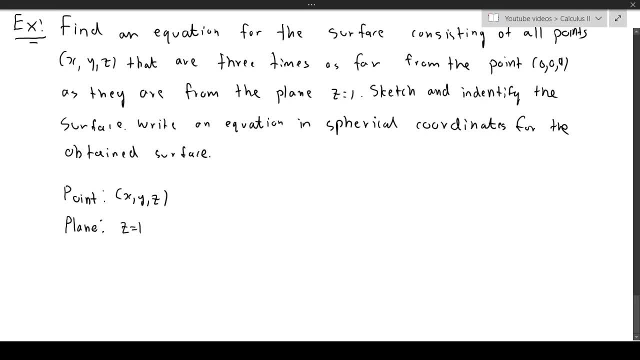 I'm going to denote this as z equals one, but then this implies that z minus one is equal to zero. Okay, so the distance from the point to the plane is d, which we derived a few lectures ago- or a few videos ago, not lectures- was ax plus by plus cz plus d. 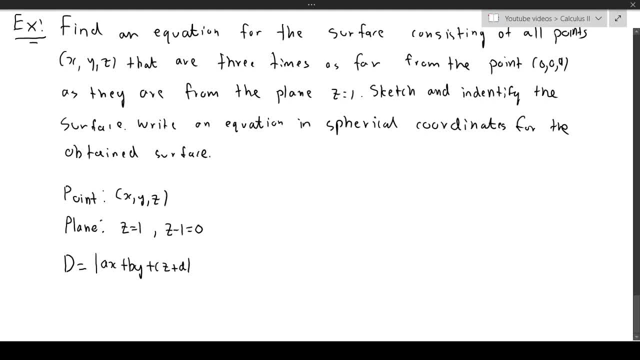 absolute value, And then we would divide this by the square root of a squared plus b squared plus c squared. Okay, so let's take a look at this. We're given the equation z equals one. Well, this means that z minus one is equal to zero, But then this implies that we have this variable here. 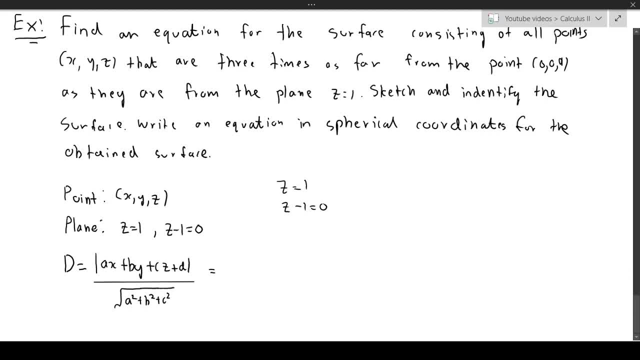 and we have this variable here, but we don't really have these other ones. So here we get the absolute value of zero plus zero and then plus cz. So this is going to be one times z or z, then minus one, over the square root of a squared plus b squared, but that's a zero and then c squared. 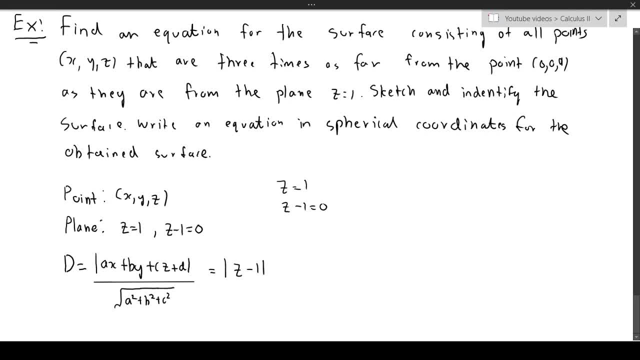 that's just one. So we get a square root of one which is just one, But then this is going to square root of one, but that's just z minus one. But then, by definition, this is equal to the square root of z minus one all squared, because we know that this 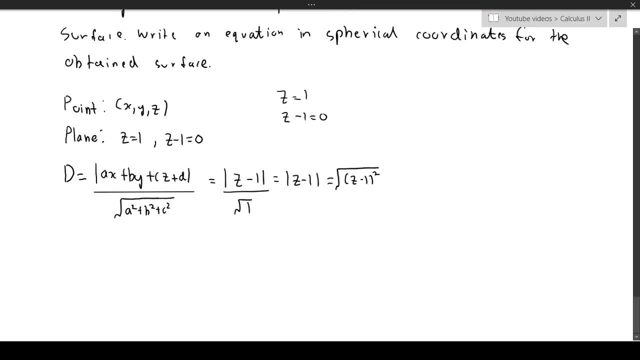 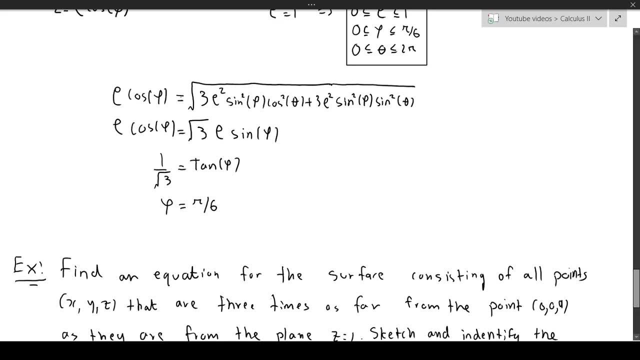 absolute value is something that's the same thing as the square root of something squared from calculus one. So this means we get the following situation: We know the distance from a point to a point is given by well, so we have a point here. 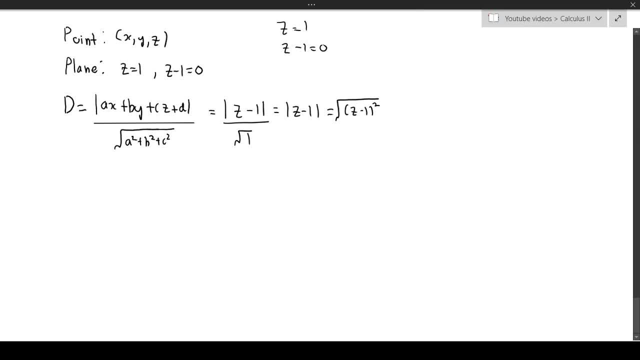 So the distance from a point to a point is given by the square root of x squared, y squared, and then z minus nine. all squared, Well, that's going to be equal to three times the magnitude of z minus one. But once again, we know that this is equal to the square root of something squared. 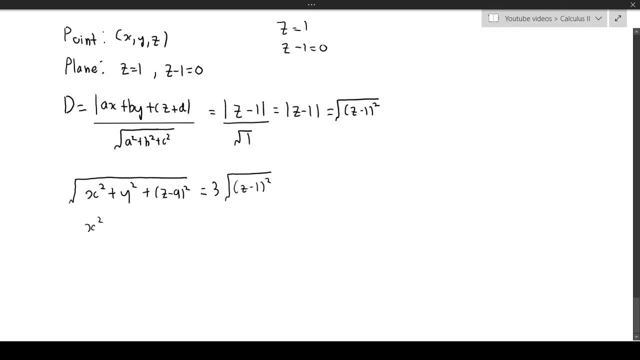 So if you square both sides, we get x squared plus y squared, plus z minus nine. all squared is equal to three times z minus one all squared. So if you go ahead and expand everything out, we get x squared plus y squared- plus or minus, I guess- minus eight. z squared is equal to. 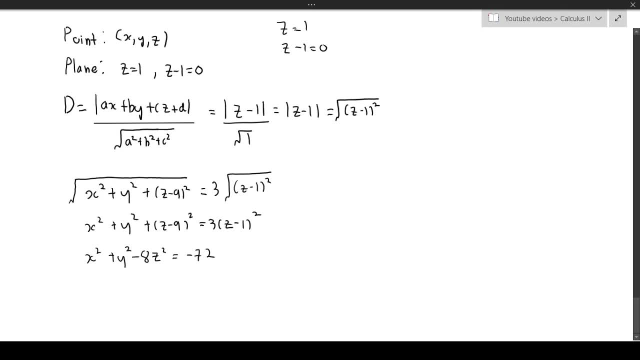 minus 72.. So that's just me simplifying and cleaning all this up. And then if you kind of move everything over, we get: 72 is equal to minus x squared, minus y squared, plus eight z squared. Okay, so if you go ahead and divide everything by 72,. 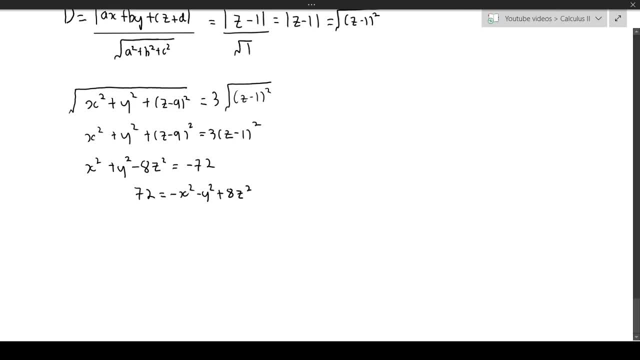 actually we can just leave it. we can leave it this way too. It doesn't really matter. But nevertheless, if you go ahead and divide this all by 72, just to get a sense of what kind of equation we have, we get minus x squared over 72, minus y squared over 72.. And then, if you go ahead, 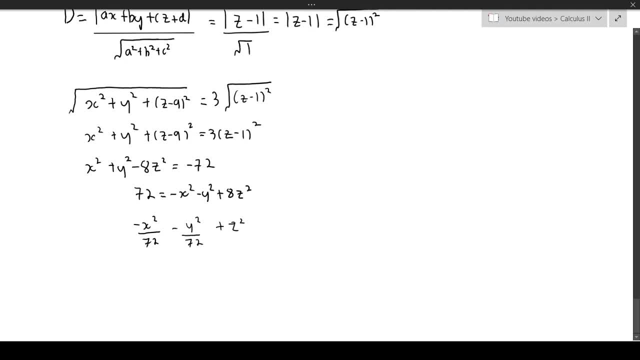 and divide this all by 72, and then plus z squared over nine, is equal to one. So that right. there is our equation. So if you go back to the video on chordic surfaces, this is a hyperboloid of two sheets. So, and the reason is because these signs are opposite. 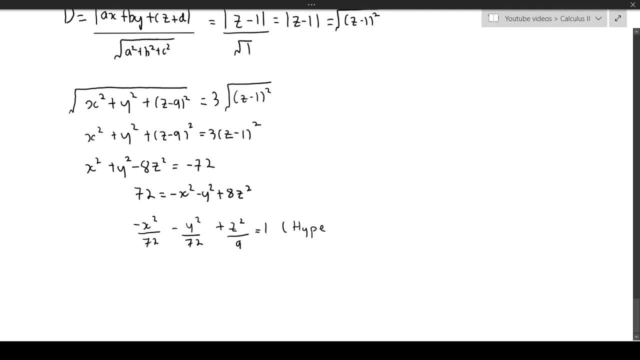 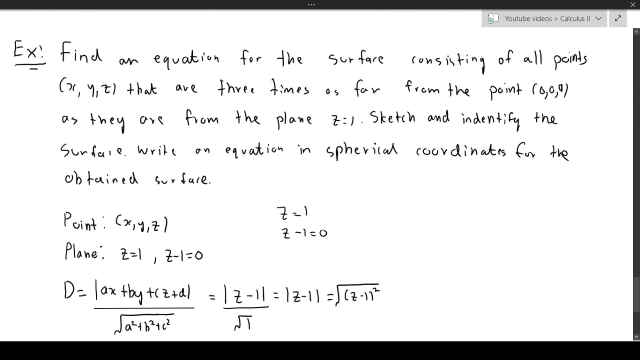 the hyperboloid of one sheet. So it's a hyperboloid of two sheets now. Okay, so we should probably talk about how to convert this into spherical coordinates. I'm actually going to move to sketching part two. I'm just going to identify the surface. that's probably a little bit easier. I could sketch. 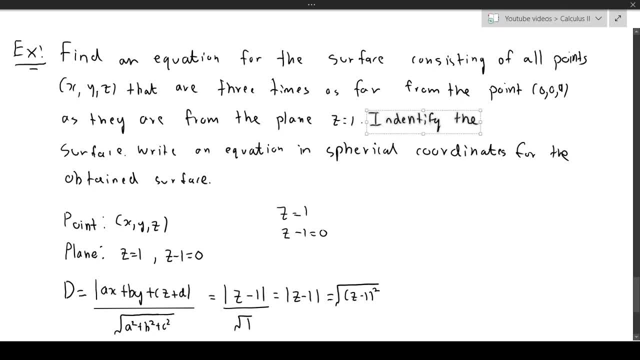 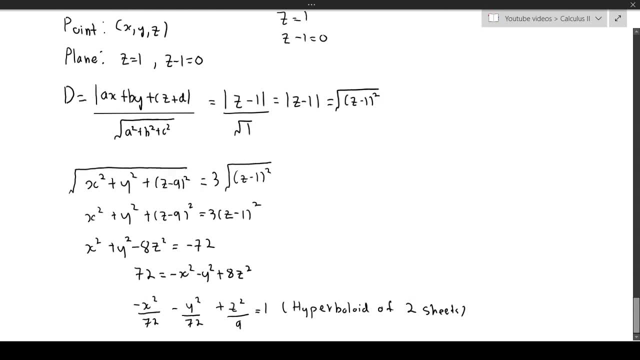 this, but 3d drawings aren't really something that's well, we can draw. we can draw 3d. It's just that it'll be a little bit cumbersome to draw it here, So I'm not going to do it here. Nevertheless, 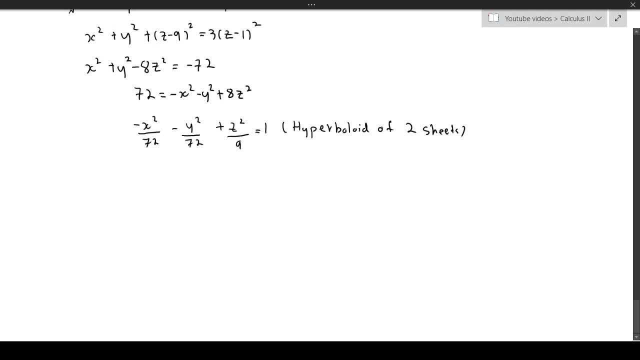 let's go ahead and convert this into spherical coordinates So we can just use this equation because that's a bit easier to work with. So if you move everything to one side, you've just kind of switched the signs around, So it's a bit easier to work with. we get x squared. 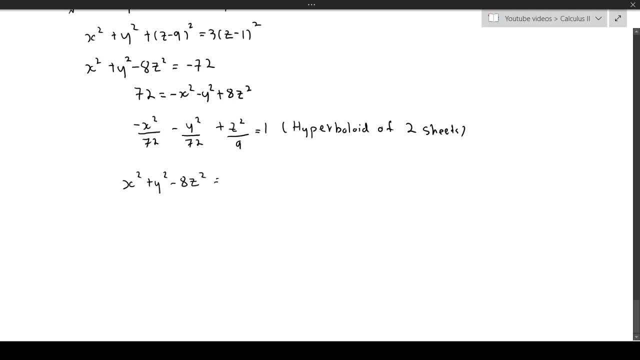 plus y squared minus eight z squared is equal to minus 72.. Okay, so now, if we go ahead and convert the x, y and z coordinates in spherical coordinates, well, we get rho squared sine squared of phi plus rho squared cosine squared of phi. 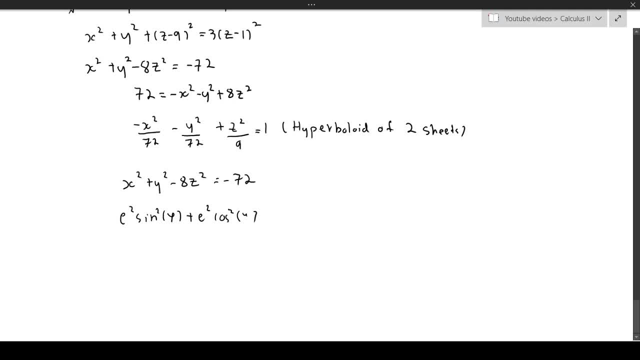 And then, yeah, Yeah, that's fine. So just to be clear as to what I'm doing here, this equation is just R-squared. So because this equation is equal to R-squared, we get R-squared minus 8Z-squared is equal. 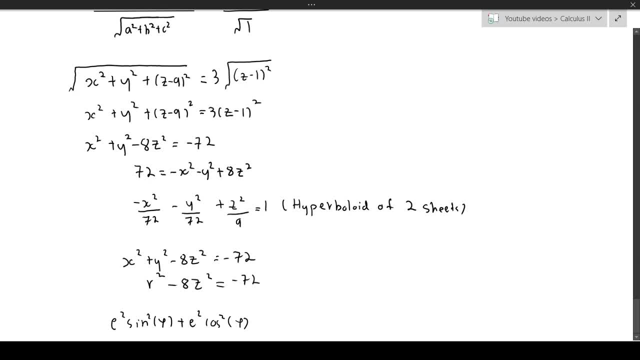 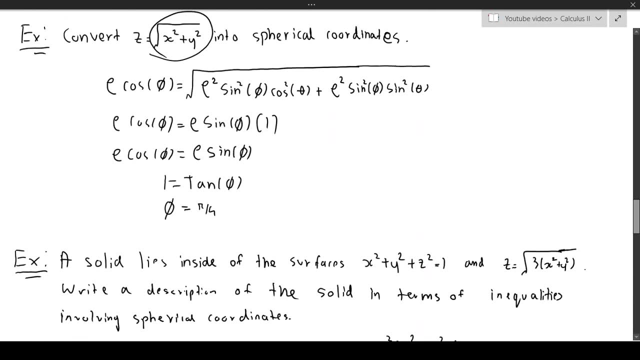 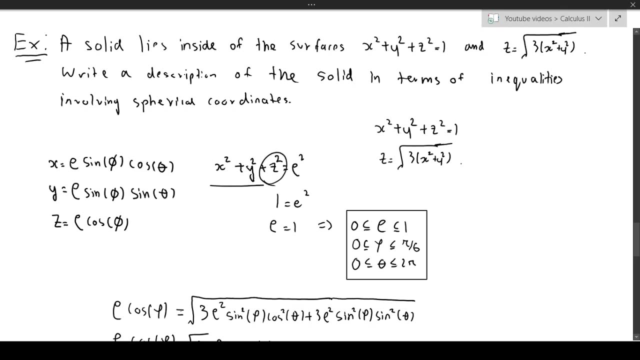 to minus 72.. And we know that X-squared plus Y-squared equals R-squared because of cylindrical coordinates as well. The row-squared portion is actually a derivation of that portion, So this part is equal to R-squared, and R-squared plus Z-squared gives us row-squared. 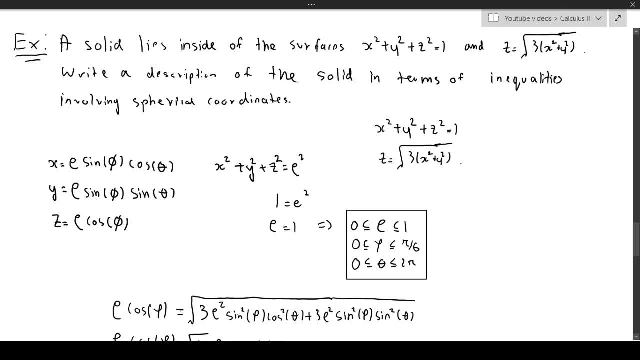 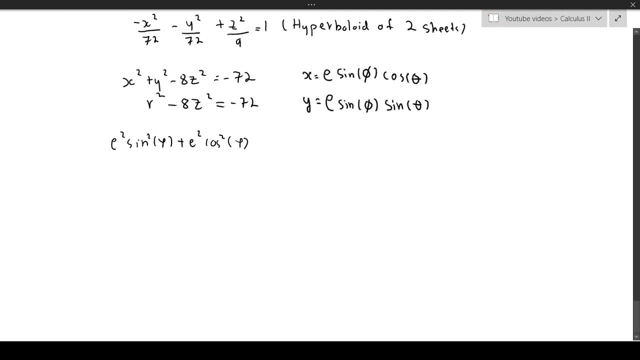 as well. So that's just the result of me deriving this using that cylindrical formula. But if you insist, you can go ahead and use these conversion formulas as well. It doesn't really matter. You look at the same thing. So, either way, regardless of however you do it, if you go ahead and plug this in for 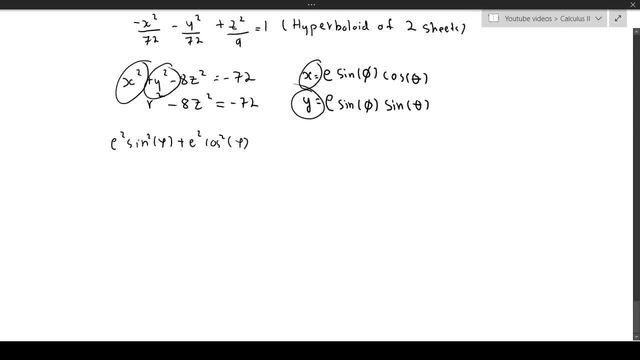 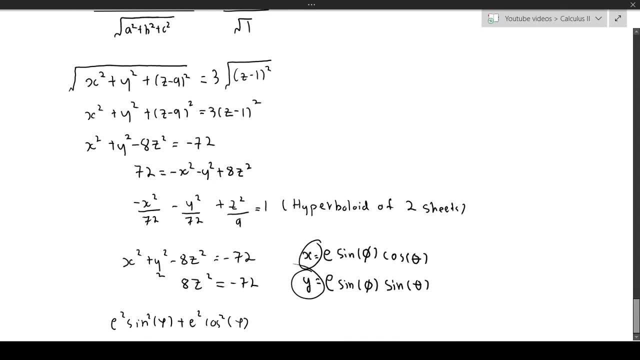 X and then plug this in for Y, you will get the same answer, So it doesn't really matter per se. In fact, let's go ahead and do that, just to give you a sense of understanding as to what's going on. 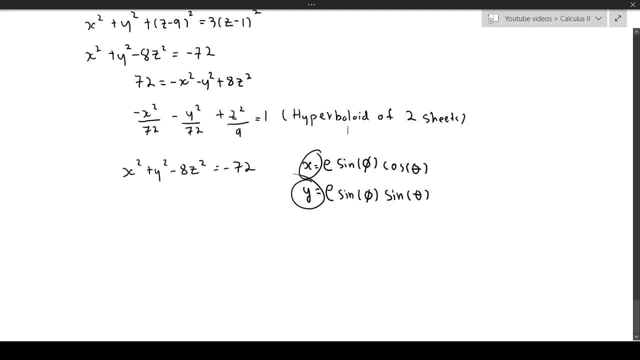 So, as I mentioned, it doesn't really matter. You'll end up with the same thing, But I think this is probably a better way of showing what's actually going on in terms of the conversions. So if you go ahead and plug this in, you'll get row-squared, sine-squared of phi. 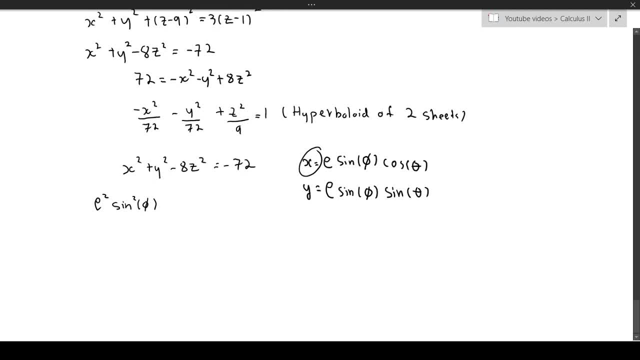 Cosine-squared of theta, And then plus row-squared sine-squared of phi, sine-squared theta. Okay, So that's what we have so far, And then we have minus 8 times Z-squared, So we get row-squared cosine-squared of phi is equal to minus 72.. 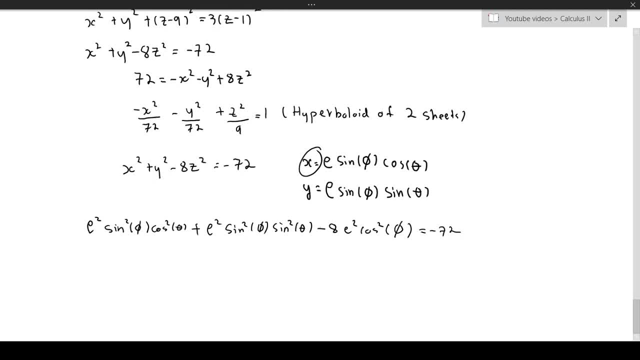 Okay, But now if you go ahead and convert this, you'll basically get the same thing. So if you go ahead and take this all out, you'll get row-squared sine-squared of phi times Cos-squared of theta plus sine-squared of theta minus 8 row-squared cosine-squared of. 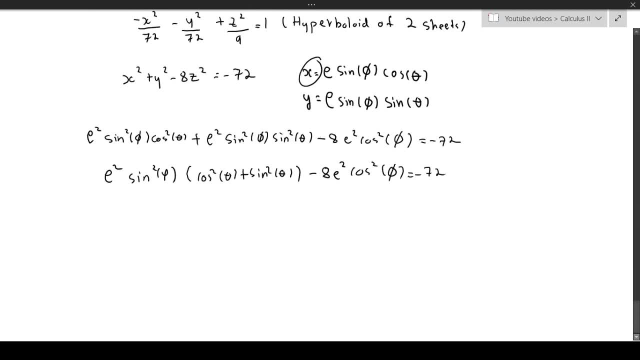 phi is equal to minus 72.. But then this is equal to 1.. So that means we are left with row-squared sine-squared of phi. Okay, And then? well, let's keep going a little bit. We can convert this cosine-squared into 1 minus sine-squared, just to make the 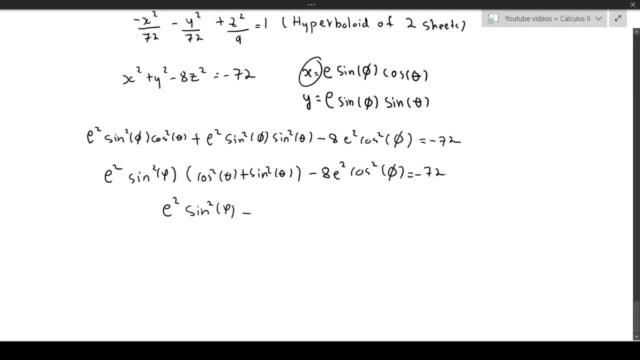 everything in terms of sine, So it's a bit easier to work with. So if you go ahead and convert that cosine-squared into sine-squared we get minus 8 times row-squared. times 1 minus sine-squared of phi is equal to minus 72..